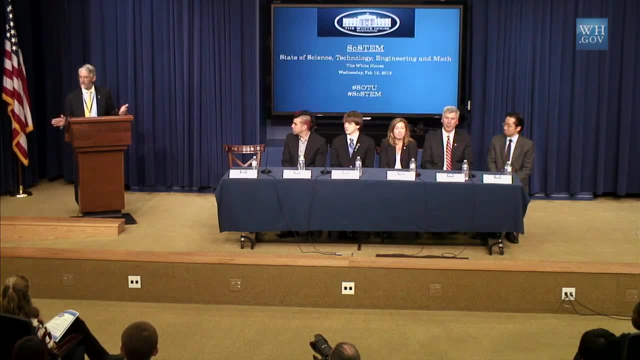 since its founding has been built on advances in science, technology, engineering and math and innovations arising from them. That was even more true in the 20th century than in the previous one, and it will be even more true in the 21st century than it was in. 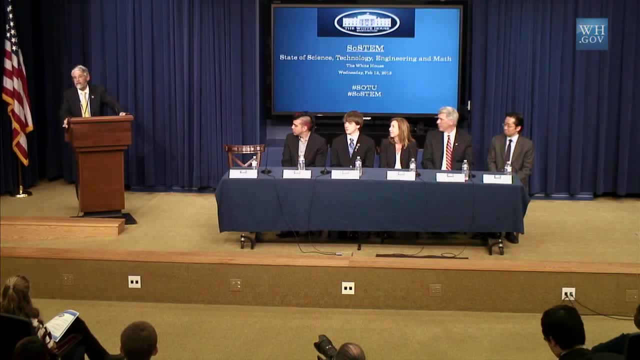 the 20th, And the result of the President's recognition of the extraordinary importance of STEM for our country's present and for its future is that we have spent a lot of time, a lot of effort, a lot of thought, a lot of resources trying to shore up, strengthen, 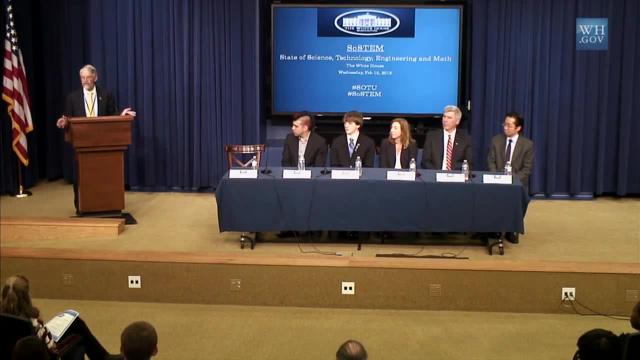 the foundations of capacity in science, technology, engineering and math and innovation in this country. And those sources of capacity of course include our investments in basic research. they include the quality of our education in science, technology, engineering and math from. 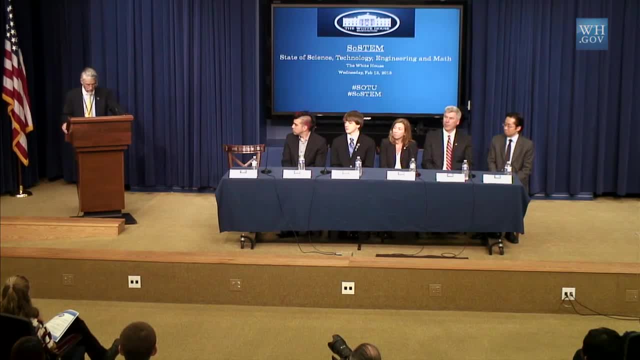 preschool to grad school and beyond. as the President himself has said, Some of the celebration of success in this domain that we have engaged in has included welcoming to the White House Nobel Prize winners, successful inventors, CEOs of high-tech companies, astronauts. 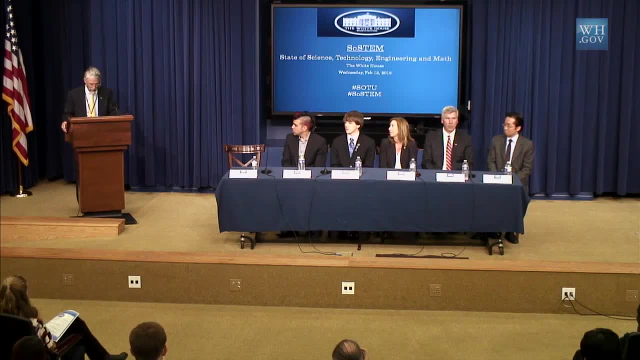 world-renowned scientists from every corner of the globe, and in fact, the chairs you are sitting in right now have previously been sat in by folks in all of those categories, some of the leaders of this country's and the world's science and technology and innovation communities, But in many ways, you are the most important set of innovators. 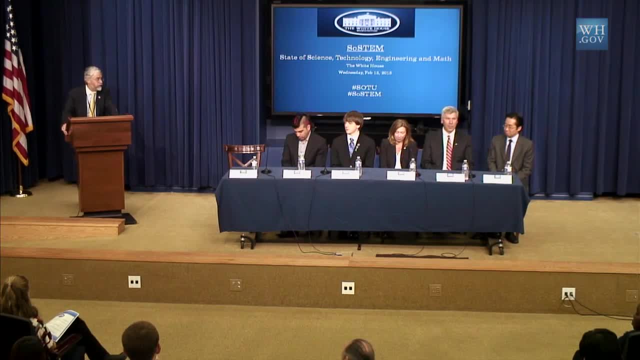 to sit in these chairs, because you are the future of STEM in this country. You are tomorrow's patent holders, problem solvers, app developers, engineers, explorers of everything from sea to air to space. You, more than anybody, are representative of the folks who are at the core of President Obama's vision. 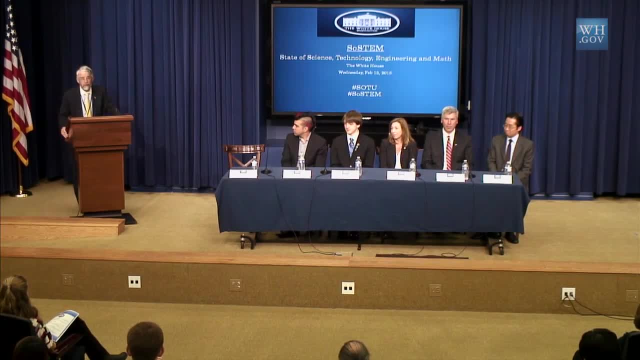 for the future of STEM in America, because you are the people who can and will turn that vision into reality. As the President has said repeatedly, science, technology and innovation are not just helpful, but they are absolutely essential to help humanity. I can speak for the entire American community, who are currently facing every one of the major challenges. 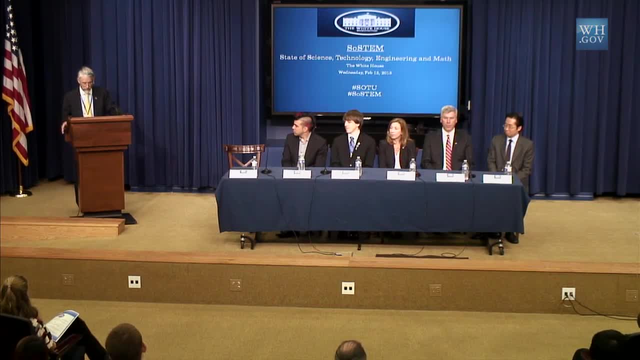 this country faces, From growing the economy and creating jobs, to protecting ourselves from natural and man-made disasters, to creating an environment in which Americans can live longer, healthier lives, to addressing big challenges like the intersection of energy and climate change, Not to mention, of course, all kinds of super exciting stuff like Monday's spectacular launch of a new Earth-observing satellite, a top-of-the-line satellite. 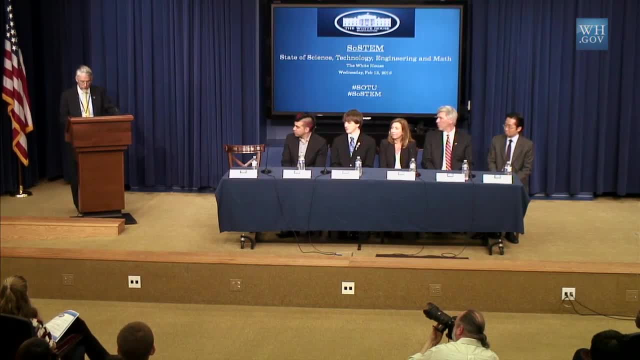 and the launch of a new Earth-observing satellite, And so those things are all an opportunity for us to be able to create a new space for ourselves. Thank you, observing satellite atop an Atlas V rocket or our plans to visit an asteroid. 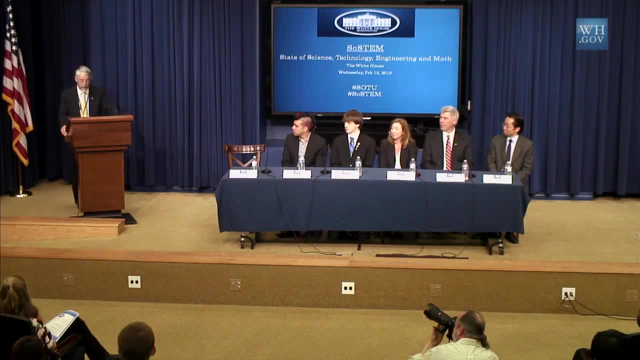 to actually take US astronauts to an asteroid Never happened before. In fact, US astronauts have never gone beyond the moon, but we will go beyond the moon and ultimately we will go to Mars. Every one of these goals has at its core some big 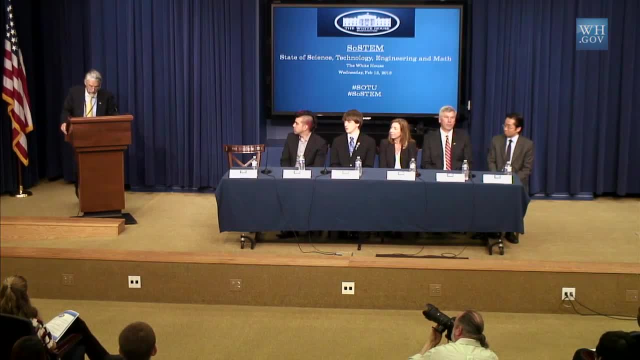 big challenges. Sometimes we call them grand challenges, But where others see difficulties as daunting mountains, obstacles, scientists and engineers see possibilities that, with the right tools and the right know-how, can become game-changing solutions. Now, this is not the first time we've invited students to the 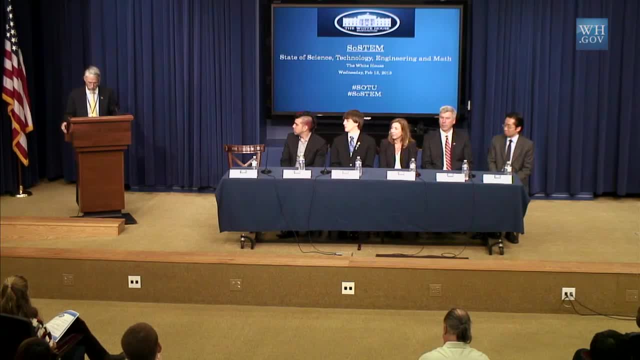 White House to talk about STEM. As you may know, the President has hosted not one, but two science fairs at the White House, something no President has ever done before. Those science fairs have invited the winners of competitions in science, engineering, math, robotics from around the country. 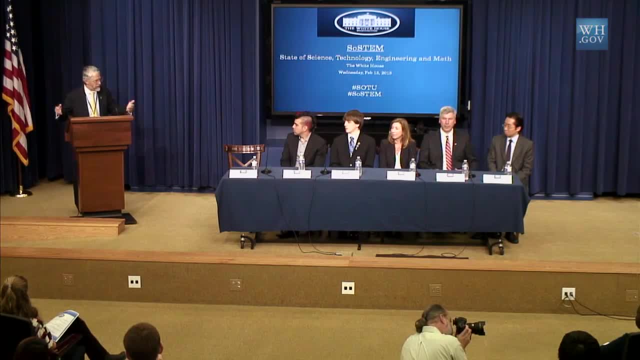 to come and present their winning demonstrations, their projects, their solutions, their poster boards, And at each one of those the President has gotten down and dirty with the kids and their demonstrations. He's prowled around on the floor with the robots. 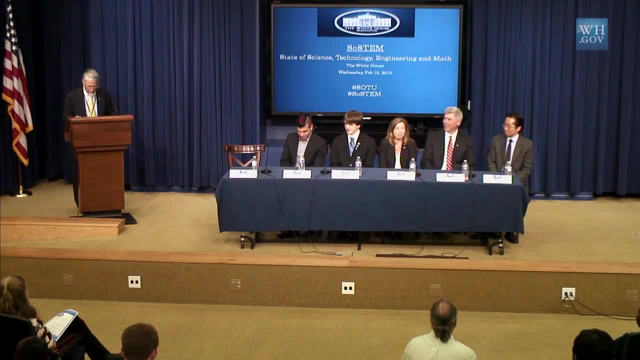 He's fired the marshmallow cannon. He has flustered his schedulers each time by spending vastly more time with the students and their projects than his schedulers had allowed, causing various dignitaries, diplomats and excellencies to cool their heels waiting for him. 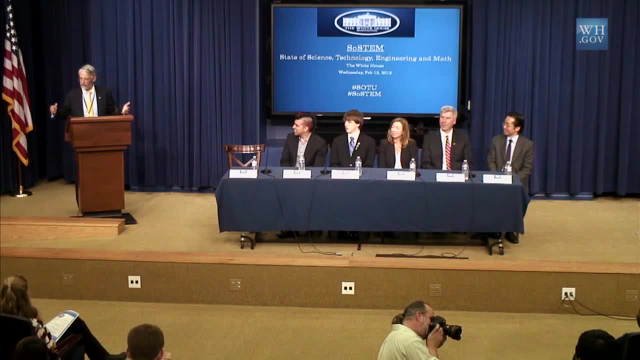 because he fell so far behind schedule in his enthusiasm for being with kids who are interested in STEM and talking about their discoveries and their excitement. If any of you have surfed the White House YouTube channel, you may even have seen a video of the President pulling the 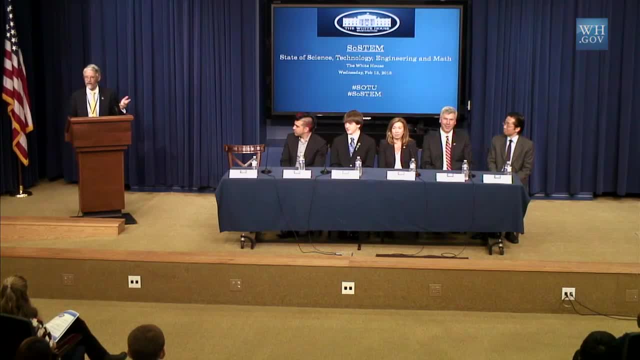 trigger on the marshmallow cannon. I have to tell you the Secret Service was not happy about that. They don't even like robots that pick things up and throw them, as was demonstrated in this room a couple of years ago when the President was standing at this podium. 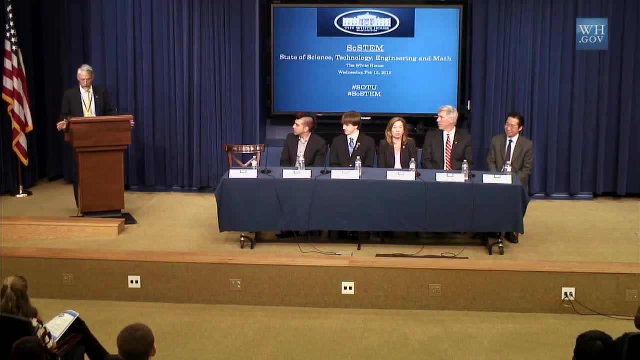 And right in front here were kids who had built a robot in a competition that involved picking up a large, rock-sized object and throwing it into a bin. It was to replicate a robot on the moon collecting samples, And it was like a three-hour argument with the Secret Service. 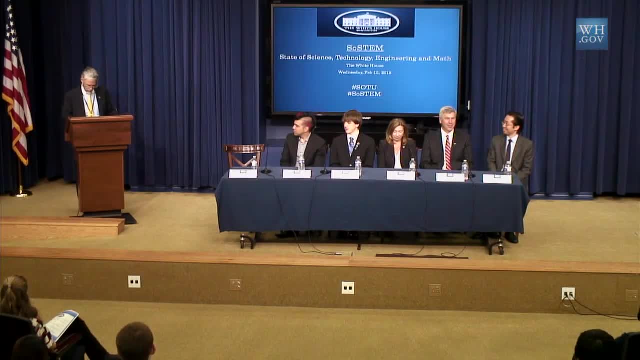 before they would allow this catapult to operate in the presence of the President, And that's what we did with the President of the United States. But we won that argument And we almost always win the argument when it comes to getting the President close and engaged with students working on. 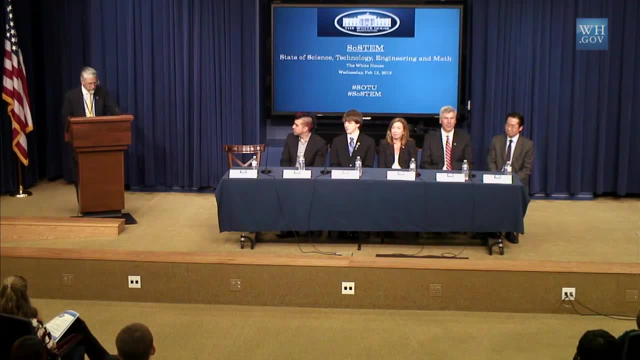 STEM topics. Obviously, we need to keep that momentum going and we plan to keep it going, And that is where you and your dedicated teachers, your supportive parents, your committed mentors come in. You're the ones who are going to keep America innovating toward. 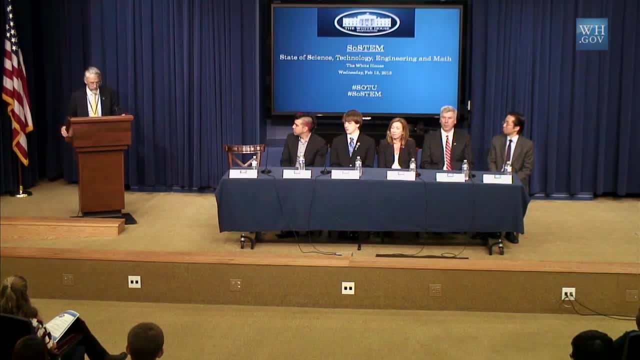 discoveries that we can't even dream about today. You're the ones who are going to find solutions to some of the world's most important problems, So we wanted to give you a chance to talk to us, And by us I mean a number of the people in and around the 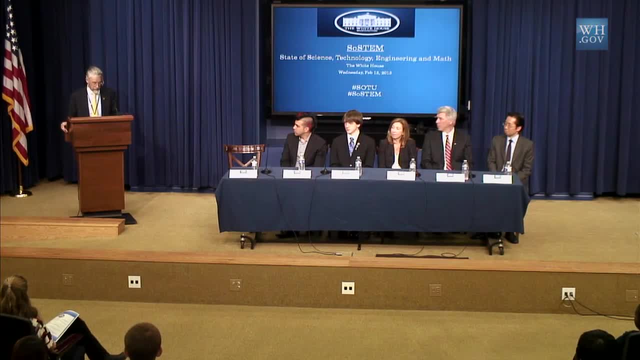 Obama administration, who are supporting our initiatives in STEM fields, including from the private sector, who are doing their share as well. So I want to introduce you to our star, our line-up here, and then I'm going to turn this over to you. 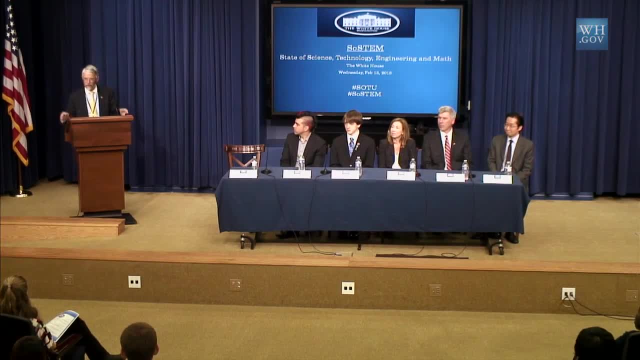 the students. We might take some questions from your teachers as well, but it's mostly about the students to tell us what's on your mind, what you care about and what questions you'd like our folks to answer. You can direct those questions, by the way. 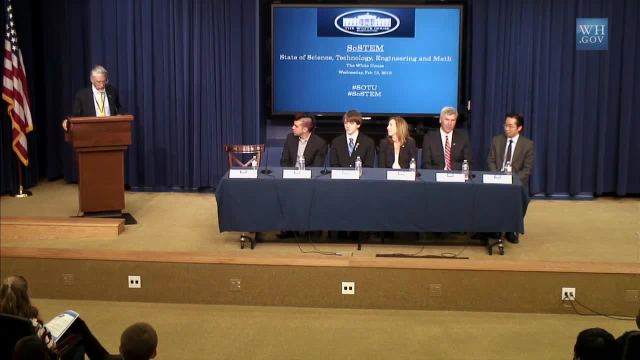 to an individual, or you can just ask me as moderator and I will try to direct your question to the most appropriate respondents. So let me introduce the panel. Starting on my far left, Todd Park. He is the nation's chief technology officer. 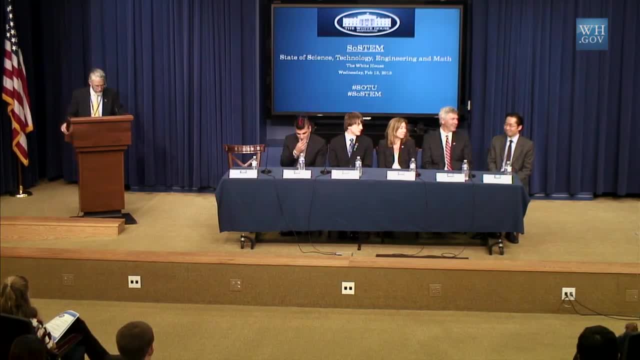 It's the first time in history that we have had a chief technology officer for the nation in this administration. Todd is a total data geek who is making sure that we're making the best use of data to spur innovation and economic growth and a higher quality of life for all Americans. 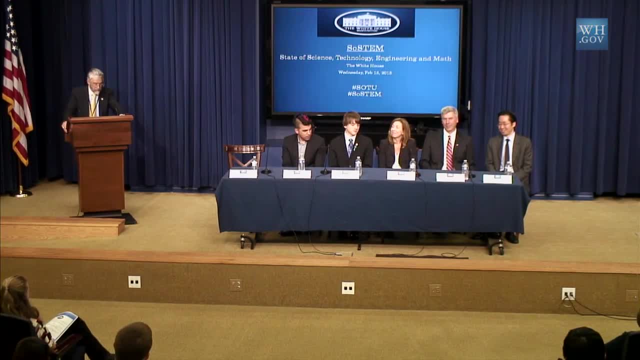 Lori Garver is the deputy administrator of NASA and has overseen a simple, simple, simple, simply remarkable array of missions into space over the past several years, as well as very important work in the domain of technology development, habitation in space, earth observation for environmental 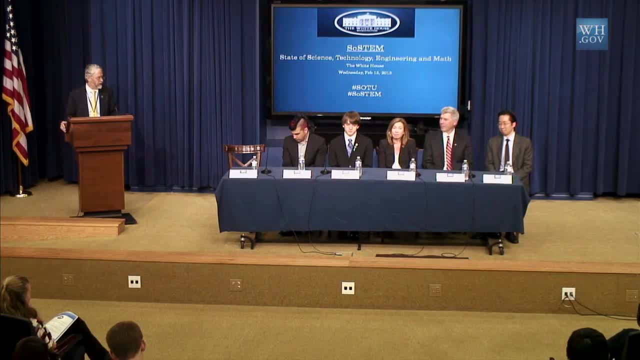 and weather monitoring. Lori is a fabulous partner for those of us in the White House in the many important domains of space. Peter Hudson, I got them quite out of order there. The chair arrangement was different than my notes arrangement. I apologize, Peter Hudson. a physician by training. 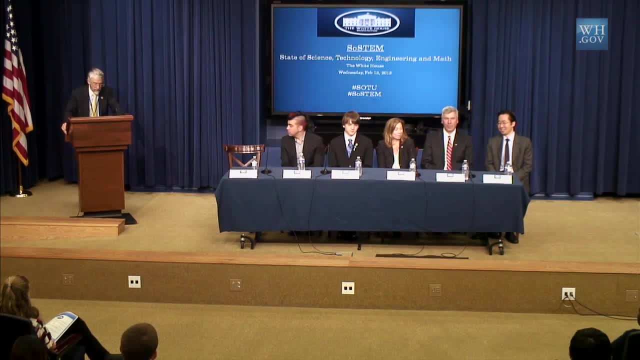 Peter is the co-founder and CEO of iTriage, a startup company that has designed apps to help consumers find the best doctors and hospitals and other health care resources for their needs, all based on data of the sort that Todd Park is making sure everybody has available to use. 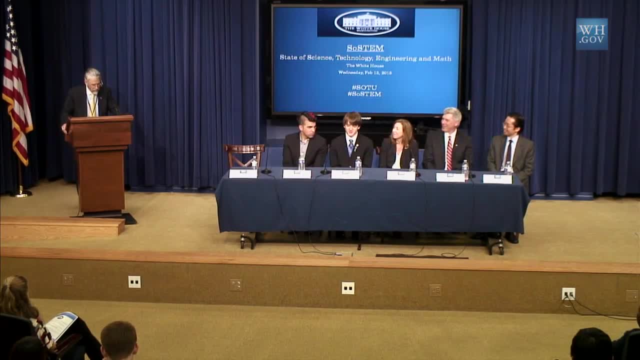 Jack Andraka, just to the right of Lori Garver, is a high school sophomore. I know some of you in the audience can identify with that. He is also the most recent winner of the Intel International Science and Engineering Fair for his creation of a new method to 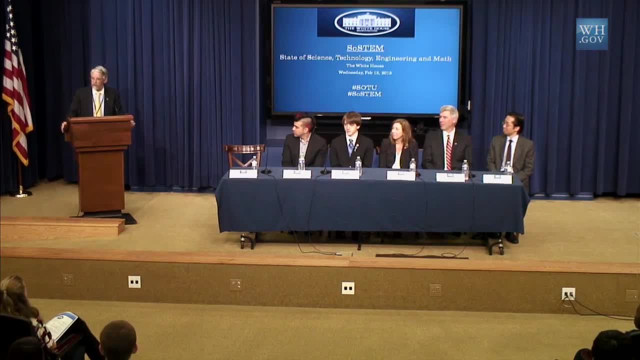 detect early stage pancreatic cancer. And I have to say that when I was doing science fairs as a kid, you know we were doing baking soda, volcanoes and things like that. It's clear that science fairs have come a long way since then. 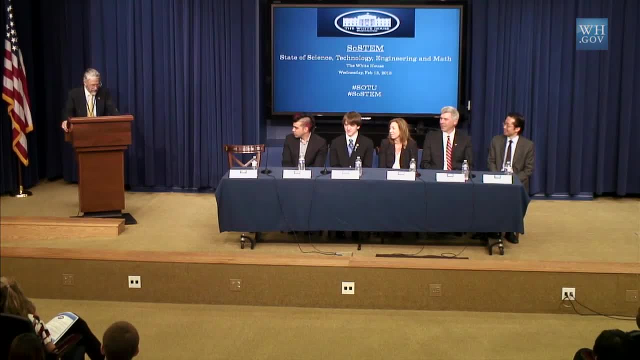 and congratulations to Jack Andraka for an absolutely extraordinary thing for somebody so early in his STEM career to have discovered and developed. And finally, Bobak Ferdowsky, better known to the public as NASA's Mohawk guy, a flight director for the NASA Mars. 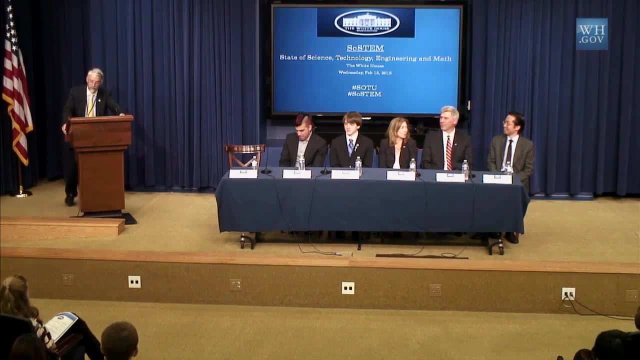 Science Laboratory mission from the Jet Propulsion Laboratory that successfully landed the Curiosity rover on Mars this past summer. I had the privilege of being in the in the building and watching that happen and marveling at the focus and dedication of all of the folks in the control room. 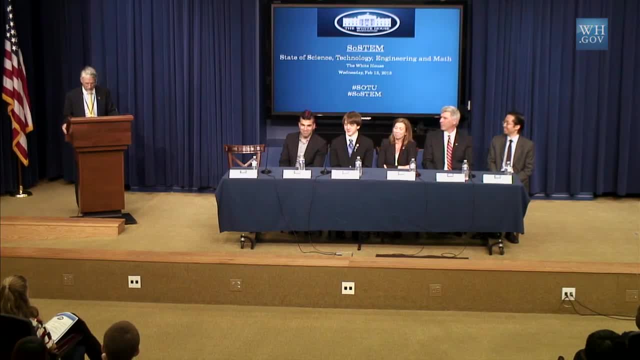 including, not least, the Mohawk guy, and we're very happy to have him with us. So, just to get started, I'm going to ask the first question. I'll ask it of Todd Park. Todd, what got you so interested in STEM in the first place? 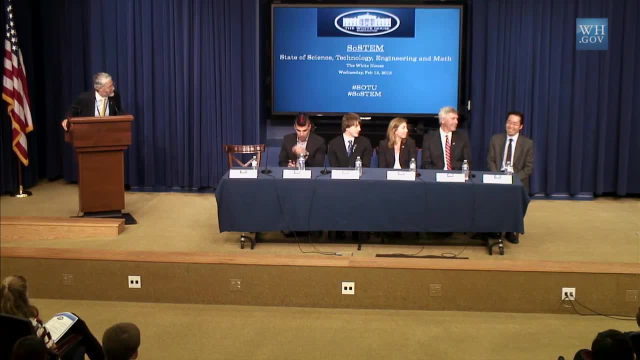 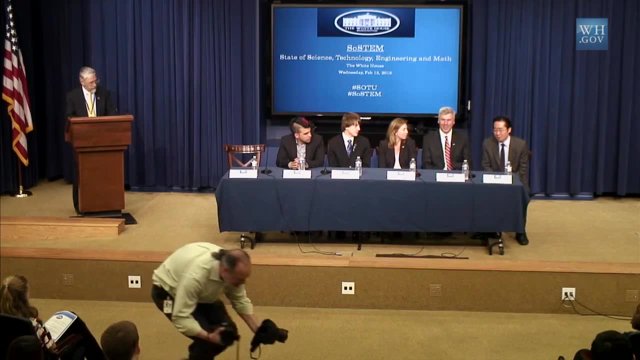 And is it true that you think data and apps are beautiful? Todd Park, Todd Park, Guilty, Absolutely believe that data and apps are beautiful. I mean, what got me interested in STEM to begin with is, I'm sure, what got a lot of people interested in STEM. 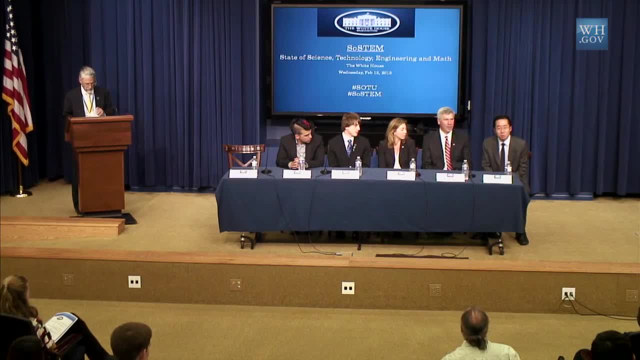 which is that, you know, it was just an incredible way to understand the truth of how the universe works. But what's actually truly caused me to fall head over heels, madly passionately in love with STEM is something beyond that, which is I've actually learned that STEM is something you can. 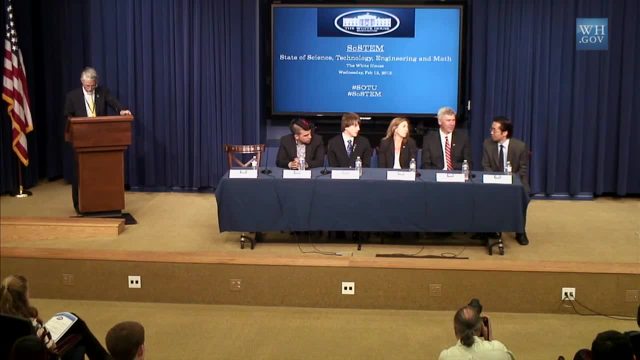 use to actually do incredible things, Unearthly things like send a giant nuclear-powered robot to another planet right, or invent a new way to fight cancer or build an app that's literally saving lives. You'll hear more about that from the panel here. 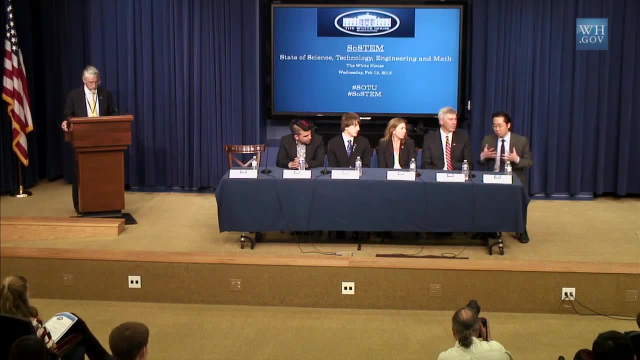 But the whole notion of STEM, not just as a way to understand the universe but to build things and do things that advance human good in almost unimaginable ways. that to me is really the magic of STEM and why I'm just head over heels passionately in a lifelong 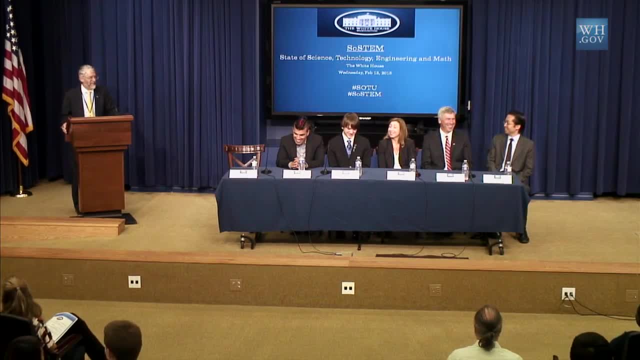 romantic relationship with it. Okay, now let's give the audience a chance to ask questions, And again, priority goes to students here. Bess has a microphone. If you raise your hand, she can come over to you with the microphone so that you can be heard. 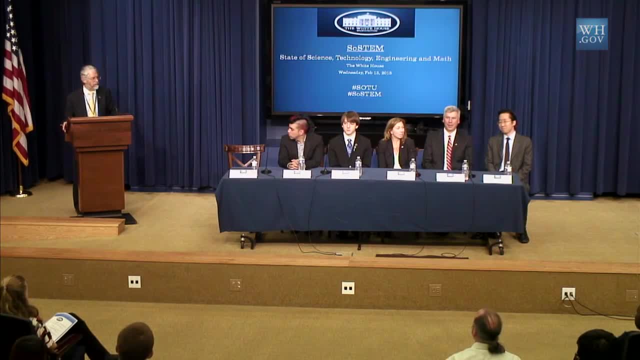 And I'd like to ask that you give your name and where you come from as you start your question. Come on, this has got to be a livelier group than that. Okay, over here. Hello, I'm Kurt Fingenstaff from Glasgow Middle School. 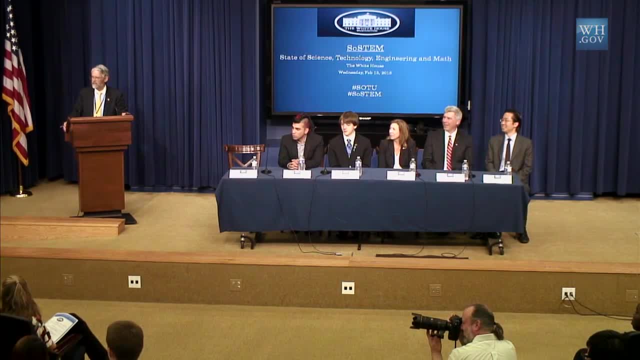 My question is: are we going to bring Germany's higher education standards to this country? Kurt Fingenstaff, US Ambassador to the United States of America. Oh wow, are we going to bring Germany's higher education standards to this country? 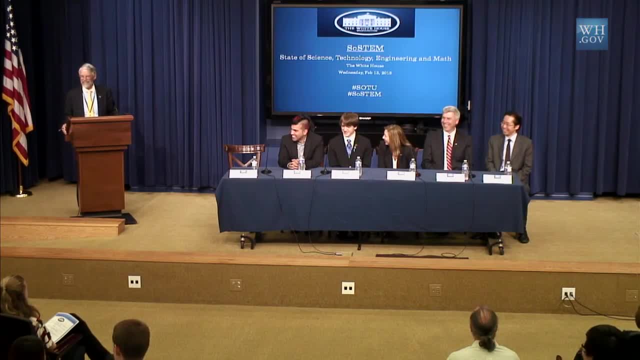 Wow, Kurt Fingenstaff, US Ambassador to the United States of America. This is a young man who listened to the President's State of the Union speech last night. Any of the panelists want to take that on? 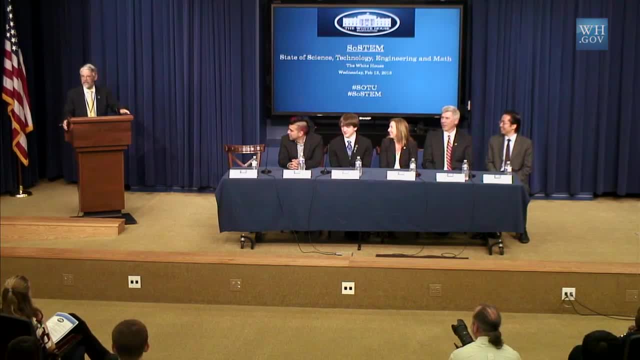 If not, I'll do it. I mean, the short answer is: you know, we're a different country, different circumstances. I don't know that we will import Germany's approach exactly, but we are completely committed to lifting our game in education. 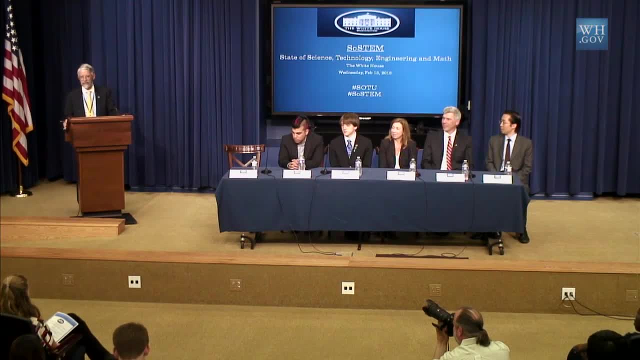 broadly in this country and in STEM education in particular. The President has said repeatedly that the single most important thing we can do for the future of our country is to lift our game in STEM education. I think that's right. We're doing well, but we need to do better. 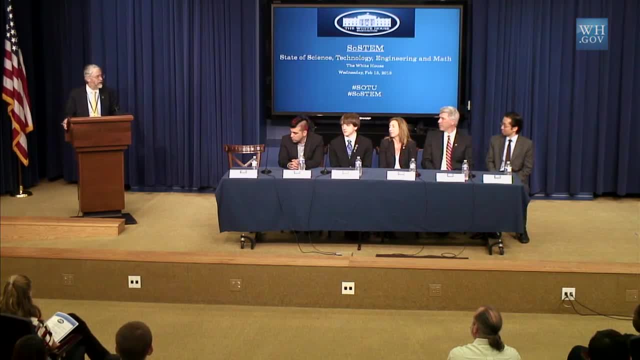 The world is getting more competitive all the time. We need to maintain our edge in science, technology, engineering and math, And we aim to develop the initiatives and the standards and the monitoring and the follow-up and the inspiration that will help us do it. 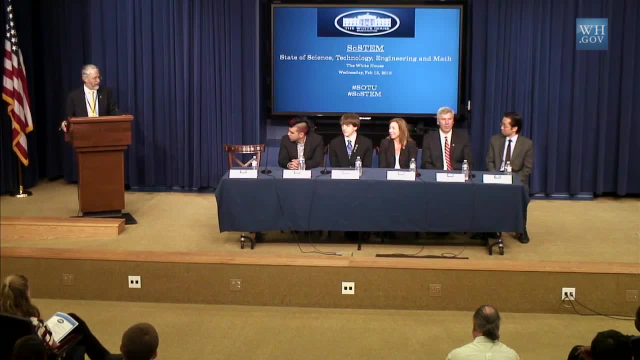 And one of the things that today's event is about is about inspiration. Science is a lot of preparation, it's a lot of hard work, but it's also all about inspiration, about being excited about the opportunities. Next question: Okay, now we're getting some action over here. 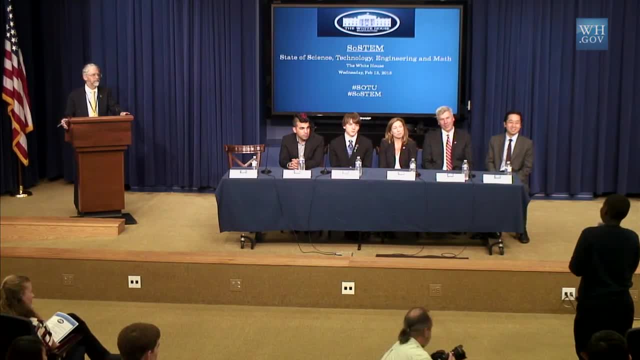 Hi, I'm Louis Campbell from Kenmore Middle School and I would like to ask Ms Garver: what is NASA's future in artificial intelligence? Ms Louis, thanks for asking the question. NASA has driven technologies across the board in all areas. 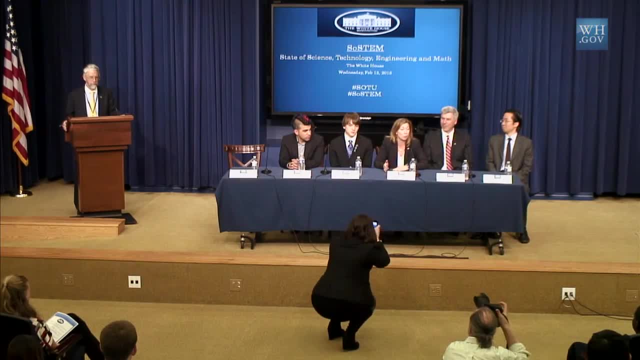 represented most recently, of course, by Curiosity, And we explore with robots that have certainly artificial intelligence, in the sense that we are not physically present with a lot of these explorers as they go out not only into our solar system but beyond. 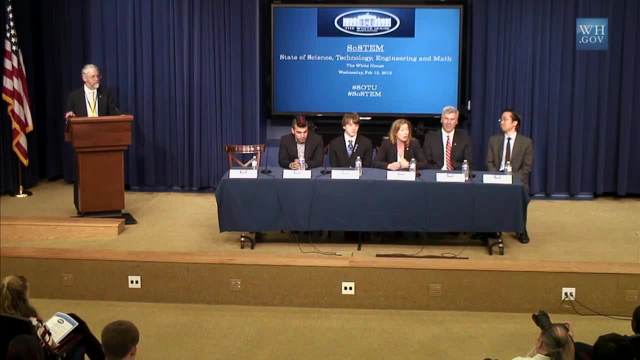 As we drive these technologies and be able to, I think, marry both the science of IT and biology- and a lot of the people represented on this panel really are doing that every day- we will be able to, I think, make advances that will benefit us. 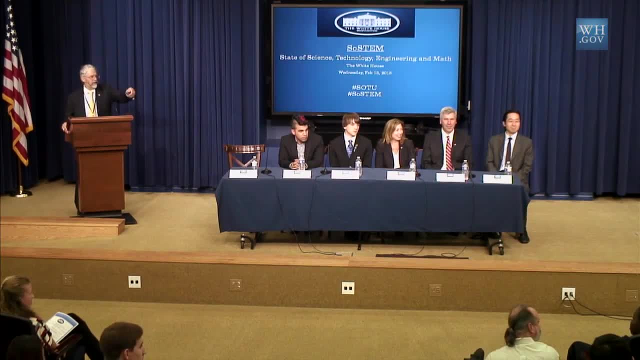 right here at home, Mr. Okay, the next one. Hey, there's one right in the second row on the edge there. Hello, my name is Ruben Dubester from Wilson High School. My question is: well, first of all, 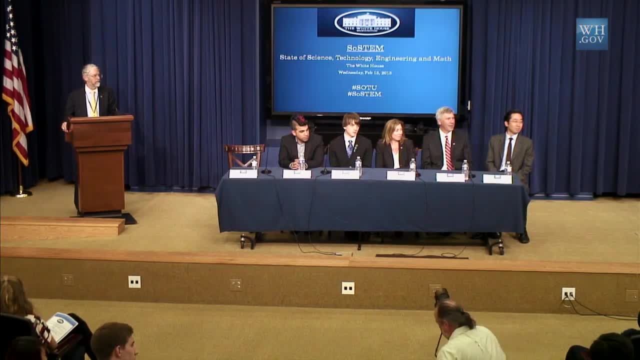 I just want to say that I deeply admire all the great work that NASA's been doing. Curiosity Rover- absolutely fantastic all that, Mr. Thank you, It was really crazy. I loved following that, But as we get on, we see that more and more private companies. 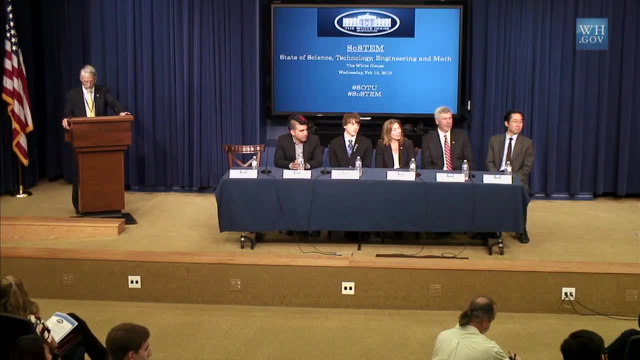 are beginning to go into the field of space exploration. SpaceX, the most famous one, flew the Dragon capsule up to the space station. Virgin Galactic is doing test flights for space tourism. So how will NASA work with these new private companies and how will that impact the future of space flight? 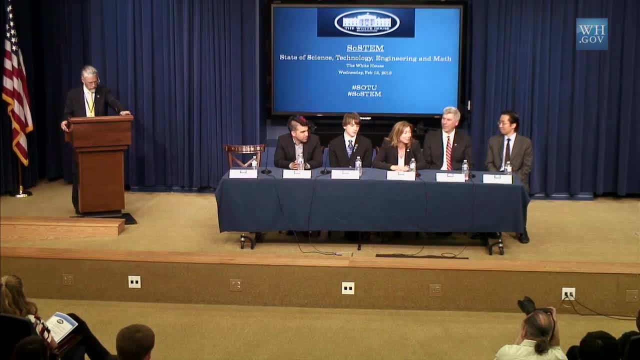 Ms, That's a great question. also, NASA has always worked with the private sector. About 80 percent of what we do is spent with the private sector. So we have 18,000 employees ourselves, but we have contractors four times that many. 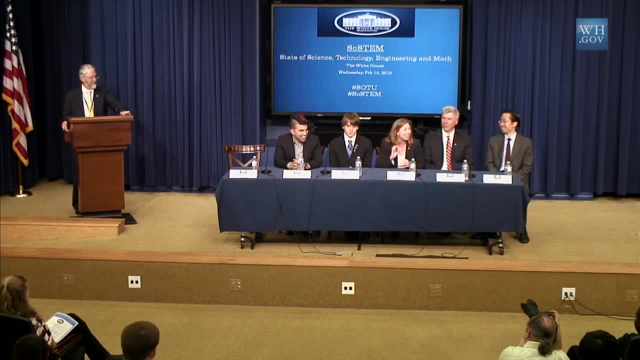 In fact, Bobak is actually a contractor, not a NASA civil servant, And so partnering in new ways with the private sector. that is another way we drive innovation, And we are looking with companies like SpaceX and Sierra Nevada and Boeing to take our astronauts to the space. 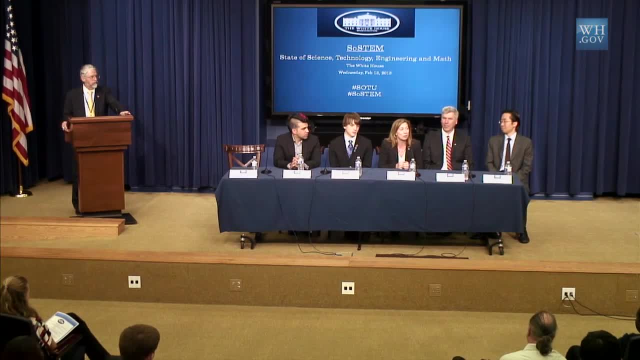 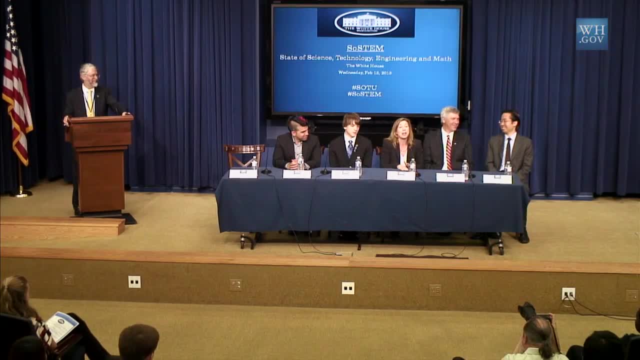 government. So the idea is we can buy a seat, but they can also sell seats to a lot of other people, And that will reduce the cost and allow NASA to invest in those things that we do best, which is exploring, driving the frontier outward and doing things going beyond. 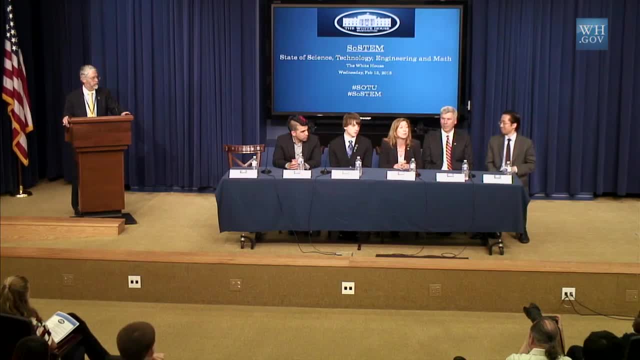 as Dr Holdren said, than we've been before to an asteroid and on to Mars. Mr Bobak, do you want to add something to that? Mr? No, I mean, I totally agree. actually, I think that that's one of the great things about the whole. 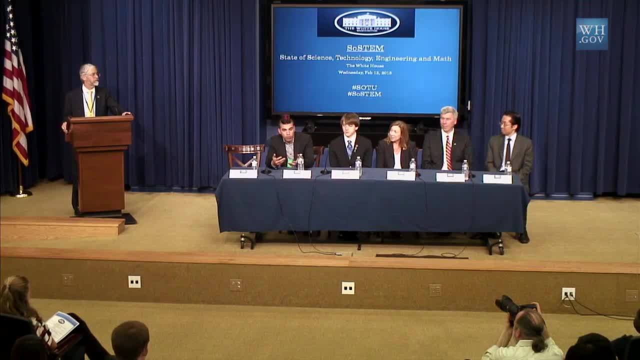 commercialization of this is that we now have the opportunity to kind of refocus our efforts on the things that we do best, and those things that hopefully excite some of you guys- Definitely excite me- is why I work at NASA. So no, I think it's an awesome time for all of us. 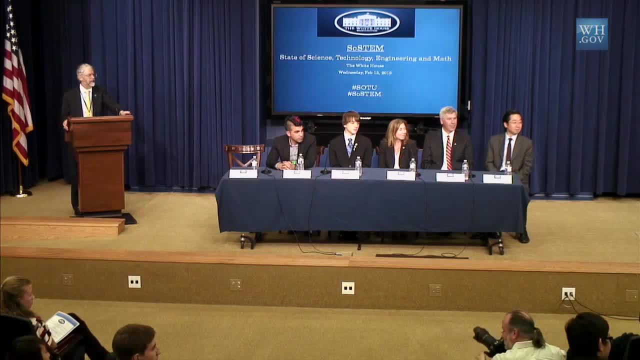 Mr. Okay, the next one. there's a woman on the edge of the third row, Ms. Oh, I'm Jania Farrell and I go to Saunders Middle School. The Press Has Curiosity: found anything on Mars besides water? Mr, That's one for Bobak, I think. 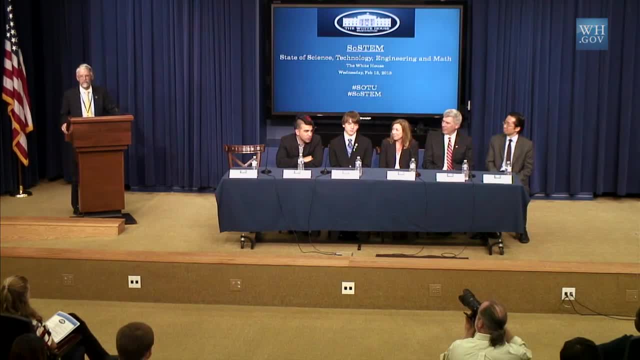 Mr. So you know, we're sort of still very early on- It's about six months in, of course, in a mission that will be two plus years. I mean, we're hoping for a decade or more. So it's kind of early to say what we've found and what we haven't. 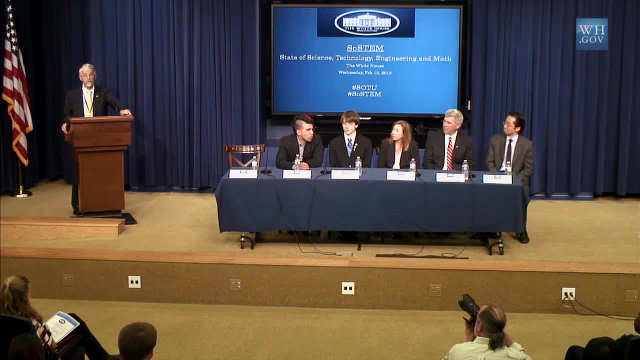 I think what we've found so far is a lot of the things that we have kind of hypothesized about Mars. we're sort of you know true so with our ground evidence, But we just did a first drill on Mars within the last week. 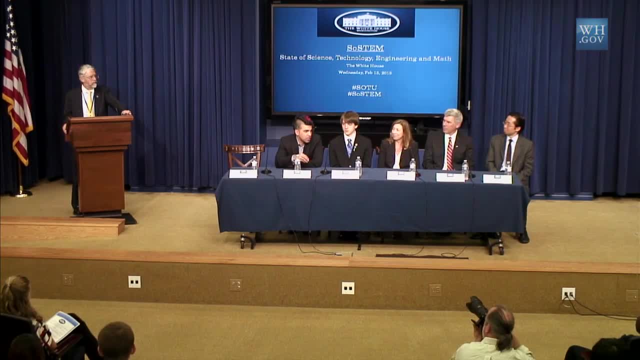 And that's actually kind of the real cool part about this mission is we're actually going to get into the history of Mars. not just the surface of Mars It's been, you know, has radiation and weathering and everything else. We're actually going to see that preserved Martian history. 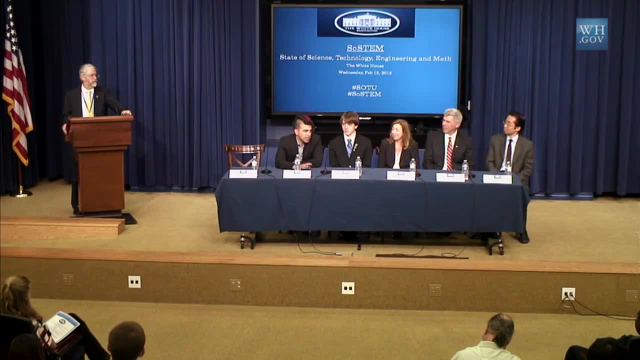 And I think that's when the really cool stuff is actually going to start showing up. So give us another couple weeks so we can actually take that sample in and analyze it and everything else. But I think it will be really cool, Mr Great. 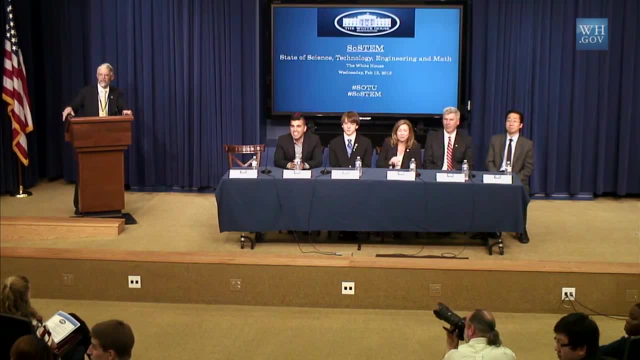 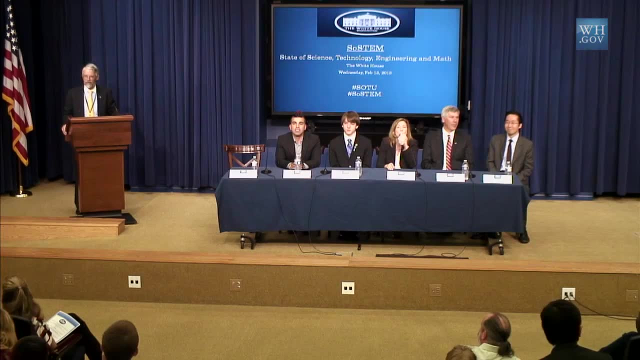 We've got to get some on. We're really missing the back. We have a whole bunch of questions in the back. Let's go back there for a while, because we've had the right side of the room has been very well represented so far. 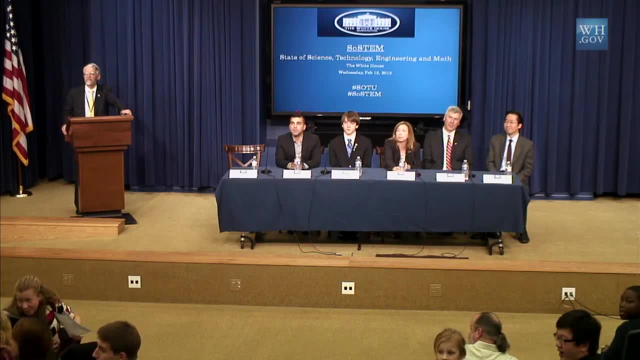 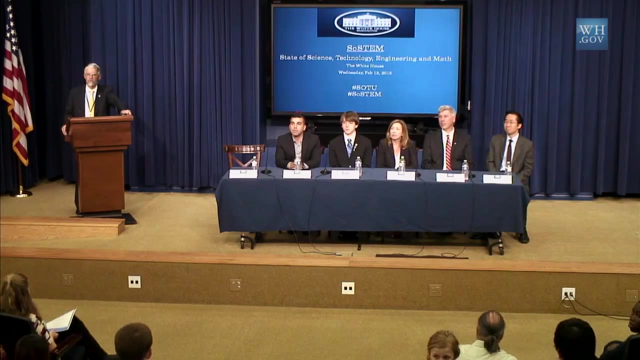 Emily Kelly. Hi, My name is Emily Kelly and I go to Thomas Jefferson High School. This is in respect to foreign language. Given the collaborative nature of science, technology and innovation, how can we better prepare students, and especially high school students, for research and 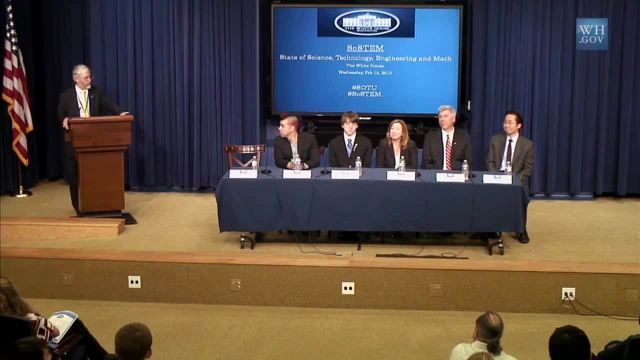 collaboration. How can we better prepare students, and especially high school students, for research and collaboration on a global level? Mr Wow, That is a great question, Mr. I'll start. Mr Bobak can start as one of our multilingual experts. 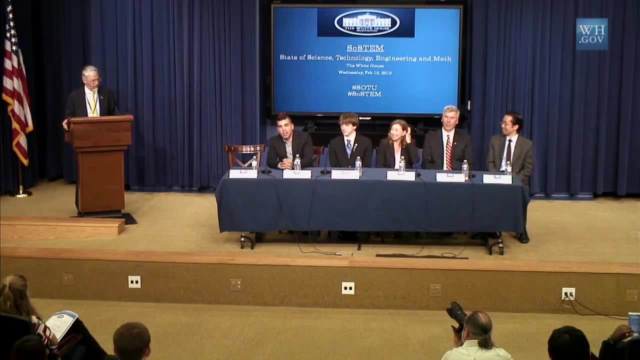 Mr No, I will say that you know, even within our mission, Curiosity, which is a very small example of this, but you know, we have instruments contributed by so many different countries: Russia, Spain, France, Canada. 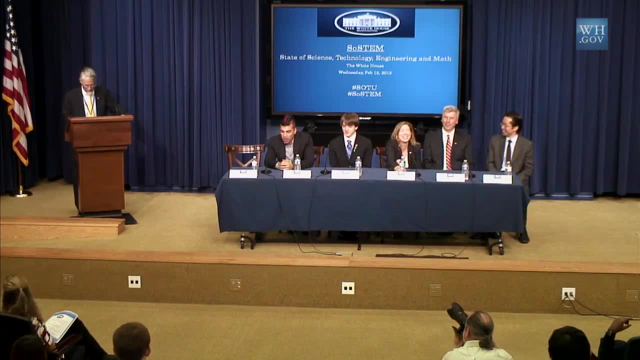 to name a few. You know, one of the things that I think is really important is that you know we have instruments that have been contributed by so many different countries: Russia, Spain, France, Canada, to name a few. You know we have instruments that have been contributed by: so 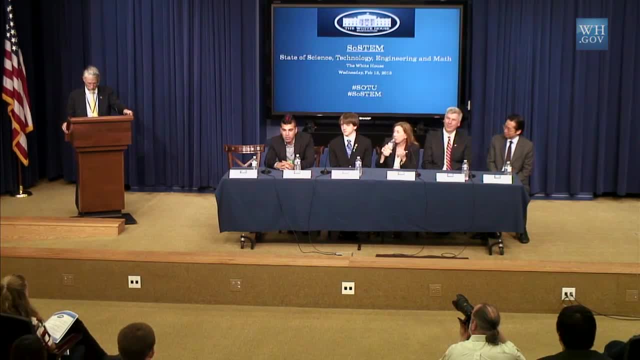 many different countries: Russia, Spain, France, Canada, to name a few. You know, one of the things that I think is really important is that you know we have instruments that have been contributed by so many different countries- Russia, Spain. 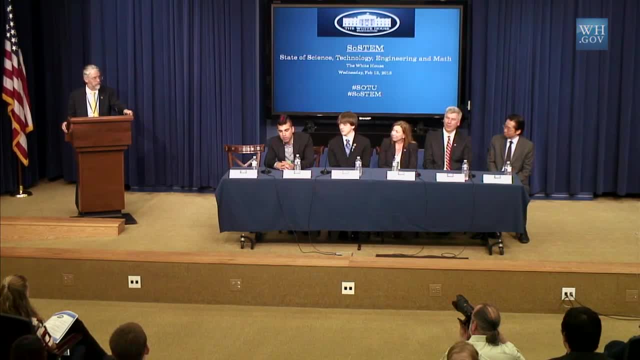 France, Canada, to name a few. So obviously a variety of languages. I mean, we tend to, of course, converse mostly in English, but I think the whole nature of what we're doing is totally going to be increasingly international, certainly for space exploration and probably for a lot of the 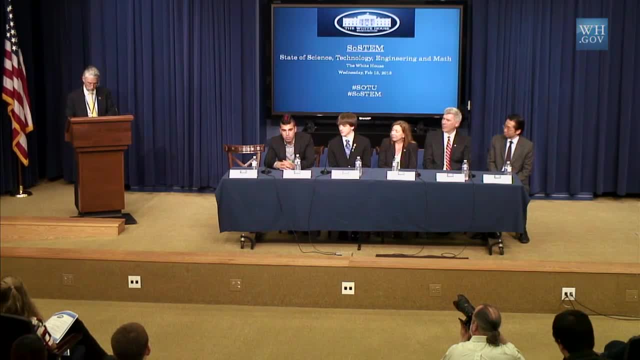 bigger challenges that, as a globe, we're going to face. So I think it's really important to actually focus it. I mean, I had the good fortune, I guess, of growing up in a multilingual household and living overseas for a while. 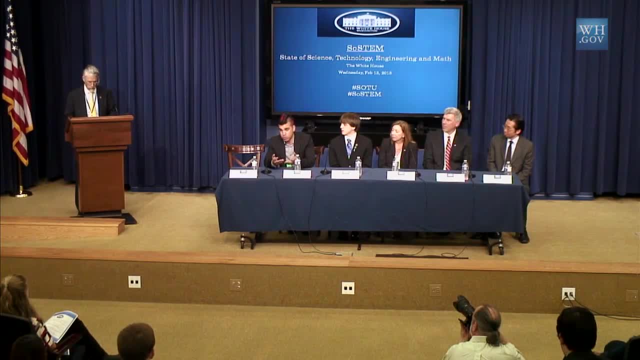 So I think it's really important to actually focus it. I mean, I had the good fortune, I guess, of growing up in a multilingual household and living overseas for a while, But you know, I would love to see that, of course. 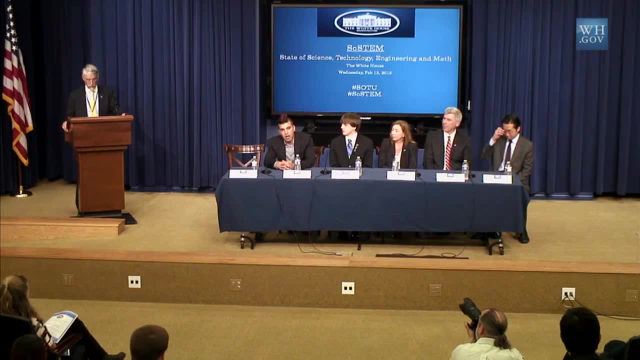 more in schools as well, to see you know a greater emphasis on that And I think it just you know, and for me personally I think it kind of helps you just approach problems in different ways, sometimes just knowing a different culture and a. 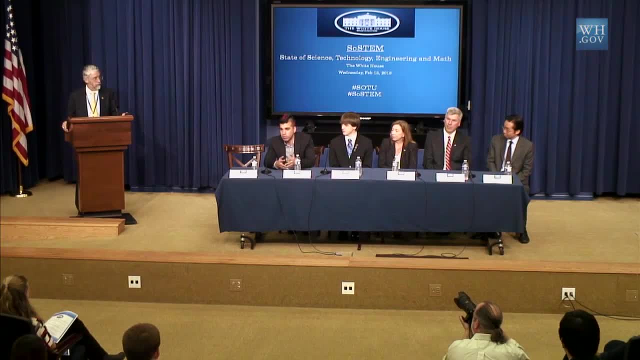 different language. It kind of helps you see things in a really different way. And of course, I do think that the role that the American people put in the work of the United Nations and other countries you know, is very, very important. 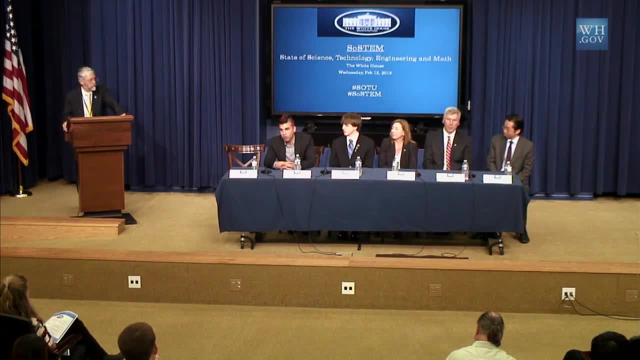 in a really different way, And that's actually a really powerful thing for STEM stuff too, because you want to be able to approach problems or even just understand where another person is coming from in their approach to a problem. Dr, I would just add to that, obviously, learning a language. 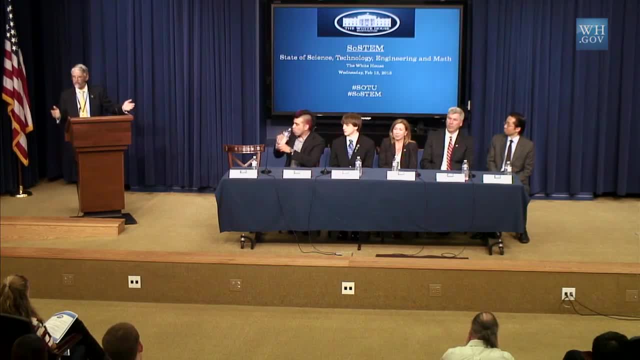 can be hard. Some languages are harder than others. Chinese is going to be a very important language for the future of our cooperation in science. It's a tough language for native English speakers to master, but it's worth it. It is famously noted that there are more teachers of English in 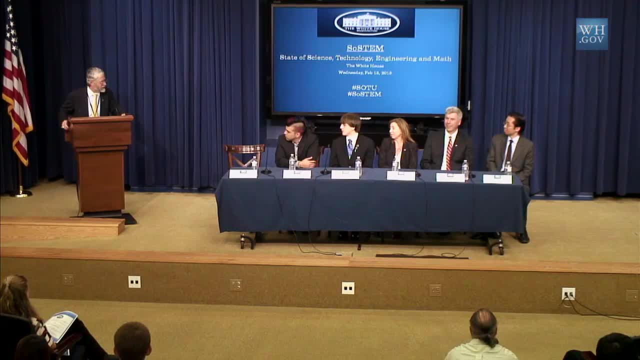 China than there are speakers of Chinese in the United States, And that is a ratio that we would do well to repair. Next question: Where are we? Where did the microphone go? We've got it back there, Okay. why don't you just work around in there? 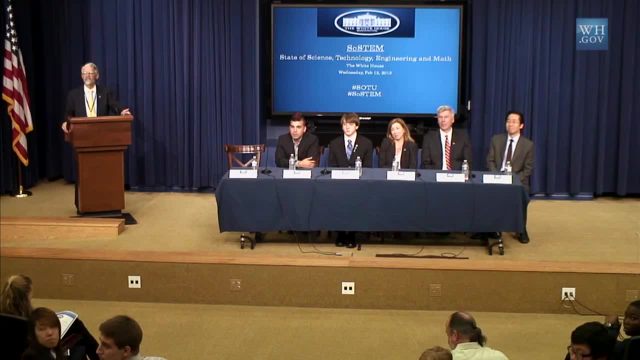 Female Speaker 1. Hello, I come from Swanson Middle School And first of all I'd just like to say, Mr Bobak, your Mohawks are really cool, Dr. Thank you, And Ms Graver, my question for you is: 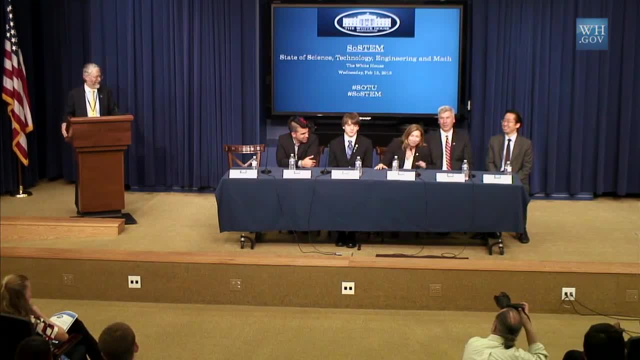 how long did it take to get to your current status, Dr? Well, I just in fact went home last weekend and talked at my high school, where I was 35 years ago. So that's how long it took from when I was your age. 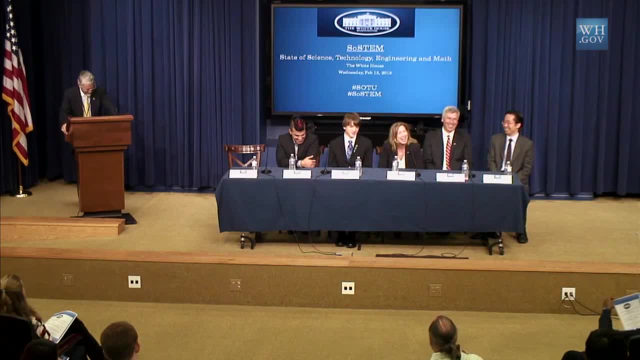 You can do the math, And I really feel that it is as really Todd Park said: growing up and asking a lot of questions and being able to make discoveries is what exploration is all about: being able to learn things that we have not learned before. that 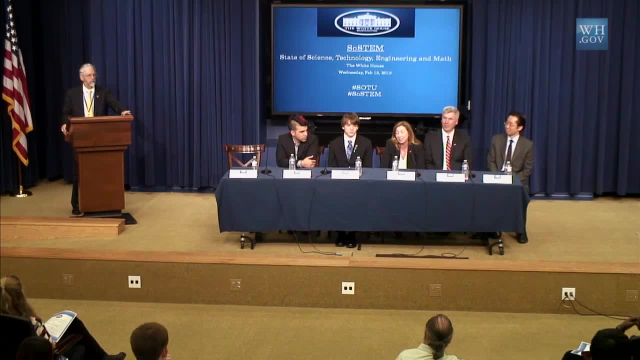 will benefit humanity and society and advance our civilization, And NASA is a place, from the vantage point of space, where we can do that. So for me it was a very exciting path that I've taken over the last 35 years. But I have. I really want to dye my hair different colors for. 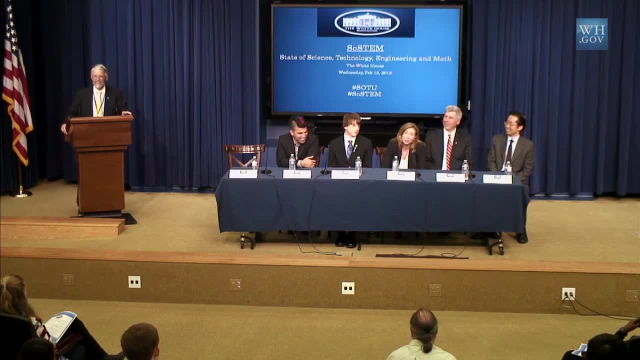 this press conference and they thought that would not be my best play, Dr. All right, Where's the mic? Okay, We have a question here in the last row before the wall. Hello, My name is Anna Voiles from James Madison High School. 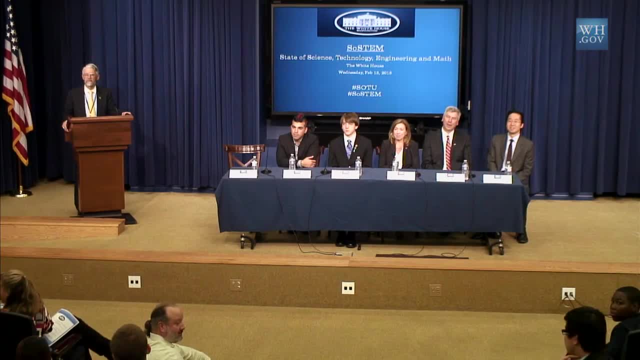 And here in the US, the liberal arts are very valued in our education system, but some educators have recently been making a push for a more STEM-based curriculum across America. So how does the Obama administration stand on that issue and also, how do you guys feel about it? 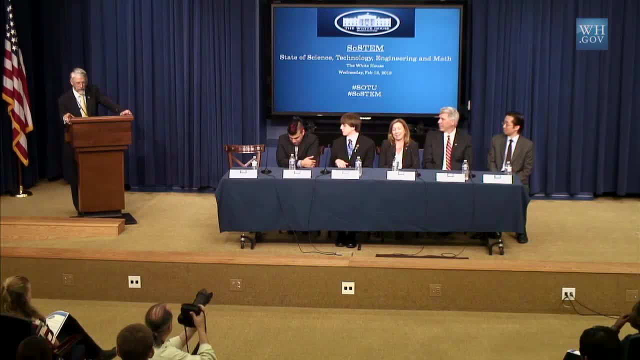 Dr. Well, I guess it depends. Well, I guess I better start with this answer. in any case, The Obama administration certainly recognizes that the humanities and the arts are important focuses in our education system: The social sciences, the natural sciences, engineering, math. 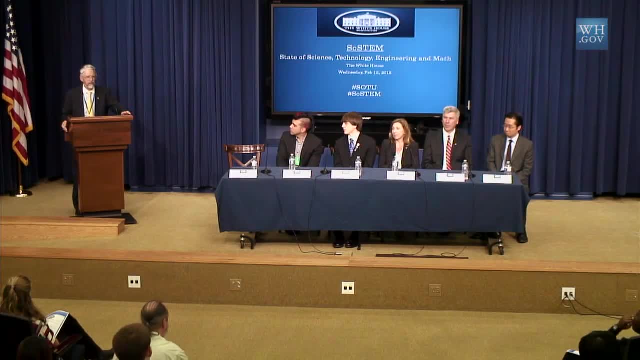 are all important focuses And our view is that people should pursue the focuses, or the combination of focuses, that most excite and inspire them and, in fact, force them to be interested in their work, to do their best work, to make their best contribution. 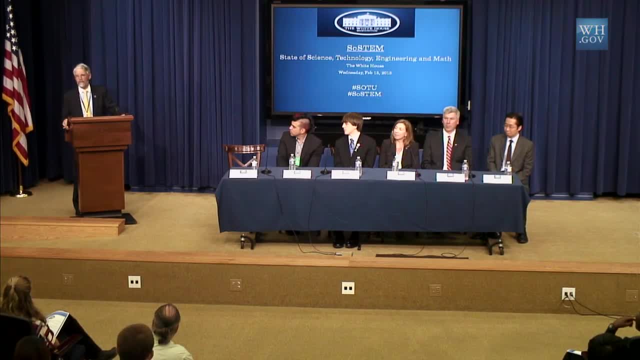 to society. Our focus on STEM has not been motivated by the view that the humanities are less important or the arts are less important or, within STEM fields, that one particular discipline is more important than another, but rather that in the competitive world, it's really important that the humanities and the arts 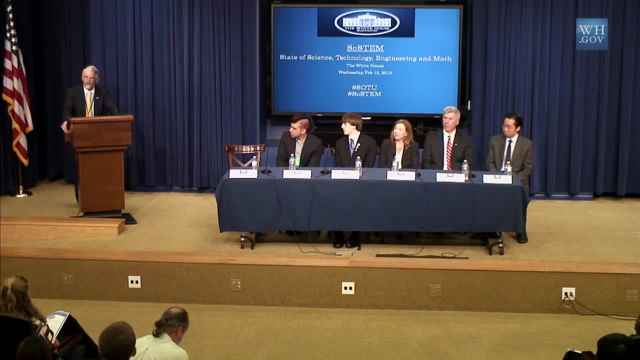 competitive world in which we now live. we have been noticing that we need to do a better job with STEM education, that this is a domain where too many kids who start out interested in STEM fields lose interest for reasons that are fixable either. the teaching is not up to snuff. 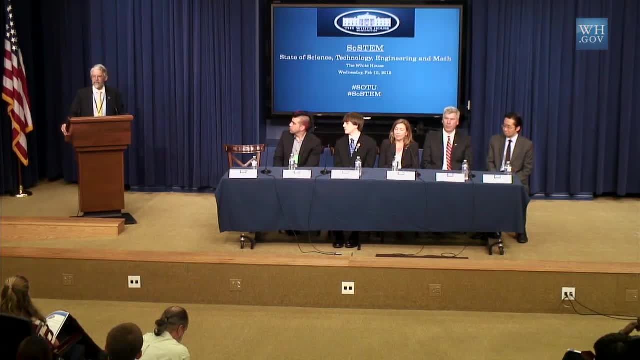 there are too many lectures and too little hands-on experience, too little exposure to the excitement and the inspiration of science and math and engineering. We don't want everyone to be in a STEM field, but we want all those who have the interest in being in a STEM. 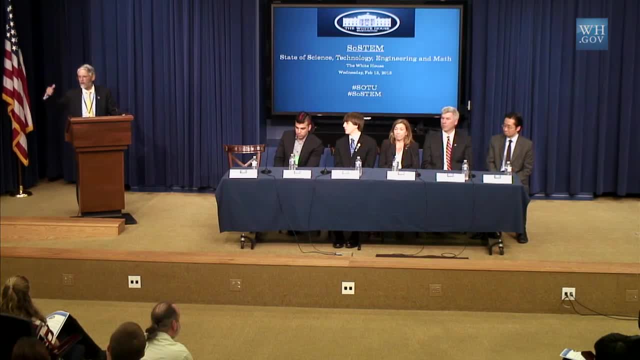 field, be able to realize their aspirations in that domain, and that requires a higher level of STEM teaching, of STEM education, than we have managed to achieve on a national basis. There are many pockets of excellence. of course, We want to replicate and propagate those. 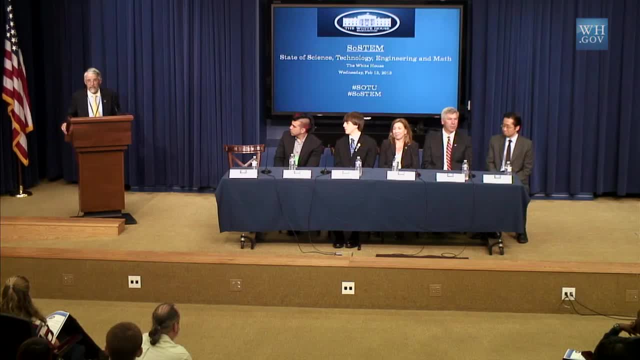 But we also want to be able to be a part of that. We want to replicate and propagate the excellence in the humanities and the arts that characterize our educational system. Let's, where is the microphone these days? Okay, so let's do some more down here. 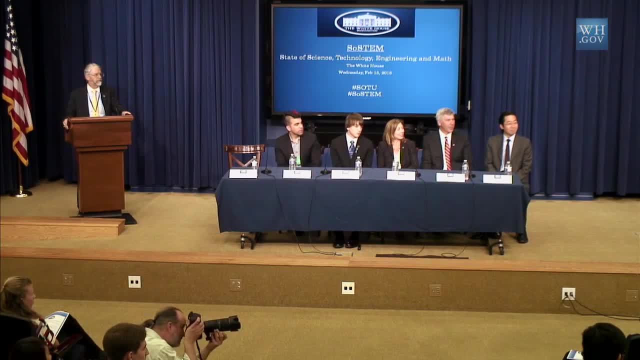 Let's go right in the front row. My name is Ritesh Raman. I come from Southwest Academy Middle School. I'm really fascinated in the field of science and technology. So how does America differ from high-tech places such as Tokyo? 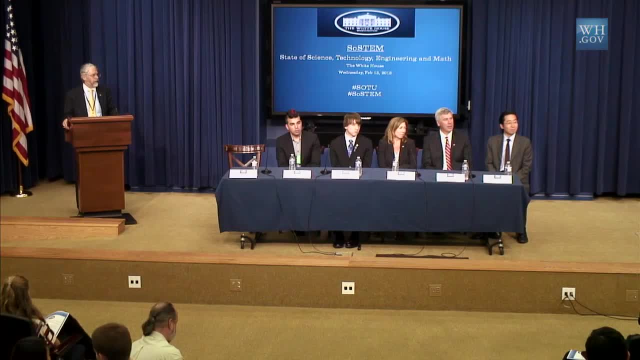 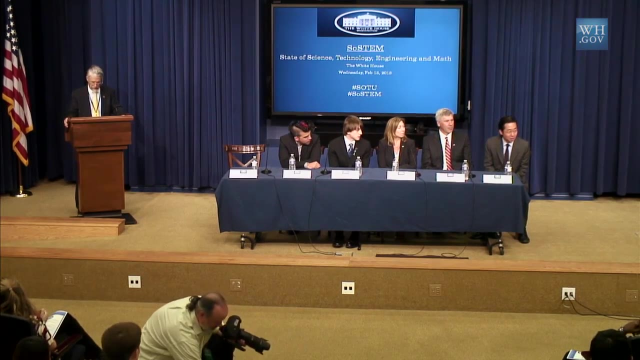 and Japan and technology- Anyone? Male Speaker 1. Hey, Todd. Male Speaker 2. Well, I think there's a lot of commonality, of course, in terms of how folks all over the world are pursuing science and tech. I actually think that one thing that really distinguishes America. 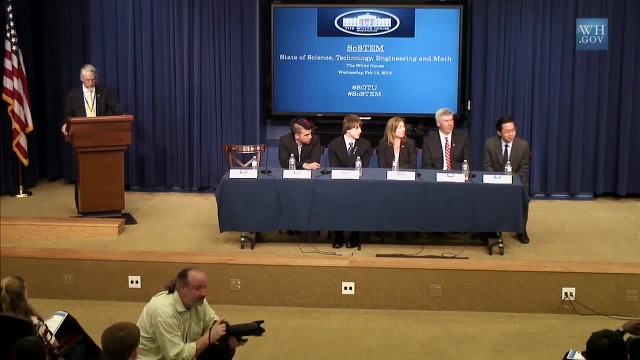 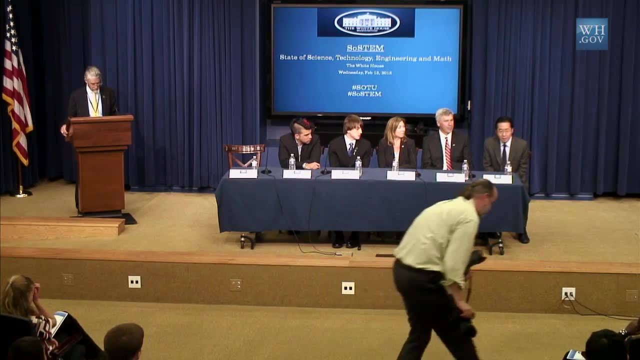 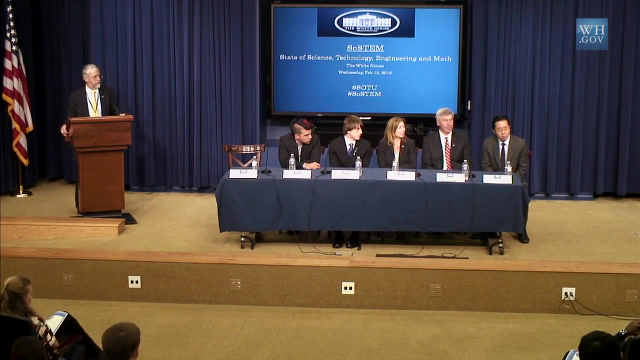 is that we take a very uniquely entrepreneurial approach to the use of science and tech. So I'm actually a private sector tech entrepreneur by background, before I actually joined the government, And Pete is an entrepreneur as well, And I think that in America you are seeing the most creative. 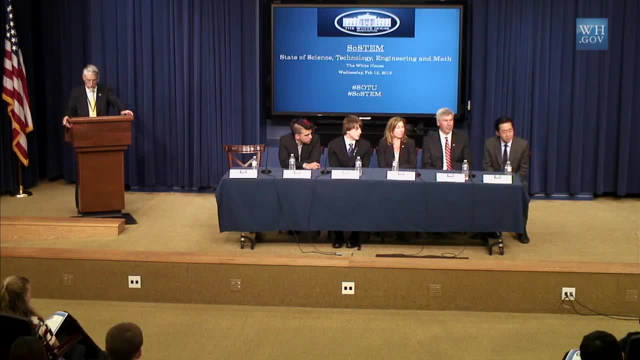 uses of science and tech to advance the public good, improve lives of Americans and create jobs. And Pete actually should tell you his story, maybe either during this or afterwards, just to illustrate that. But one of the misconceptions I think about STEM. 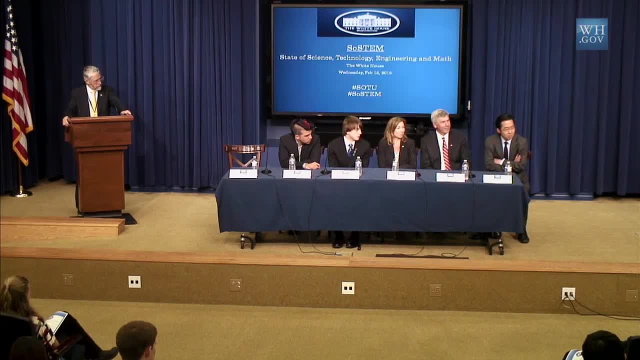 is that you know it's actually not artistic. I don't think that that's true at all. I think that actually writing a great computer program or inventing a great new machine has a lot more in common with writing a great novel or making a movie than it is sort of a. 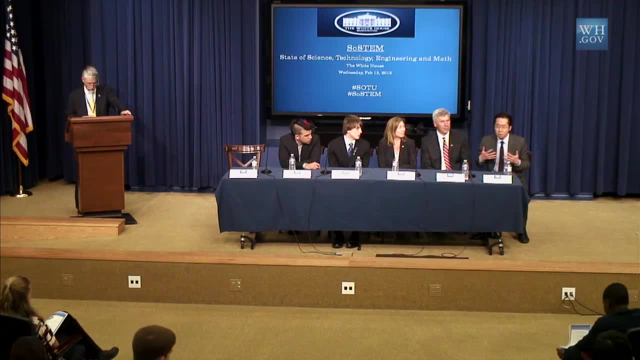 color-by-numbers exercise. And so I think actually the greatest practitioners of STEM, the ones who have contributed most to society, are actually great artistic minds, are great entrepreneurial minds. They can think boldly, think creatively, think out of the box. 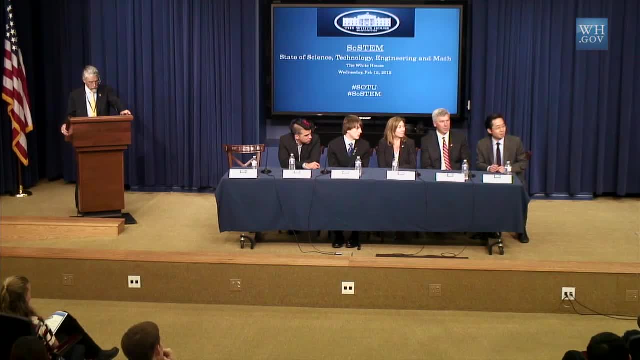 And I think- not that I'm biased, but I think a disproportionate number of those minds and hearts and souls are here in the United States of America And I think that actually there are a great number of those souls here in the audience And I'm really eager to see what you're going to do. 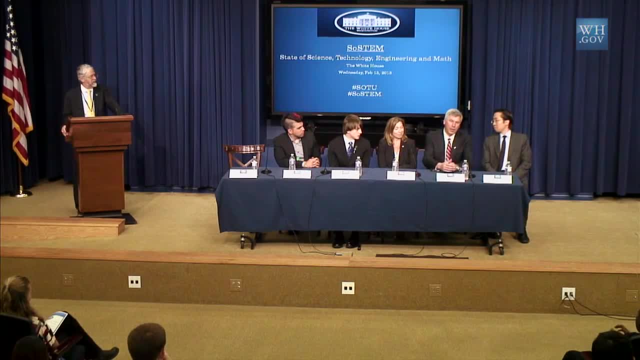 Mr Peter, do you want to add anything to that? Mr Sure, You know, I think being an entrepreneur means that there's really no road map. There's nothing that's going to tell you what your next step is. You just have to figure it out. 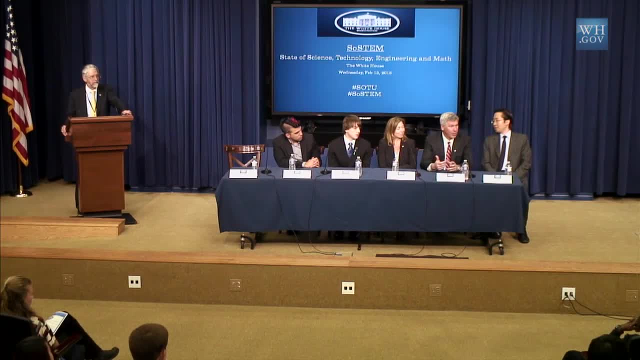 So having that creativity. you know, both Lori and I went to a liberal arts college. We learned to ask why I took Russian literature and I took pre-med. So I learned a lot of the humanities, but I also had a really good science background. 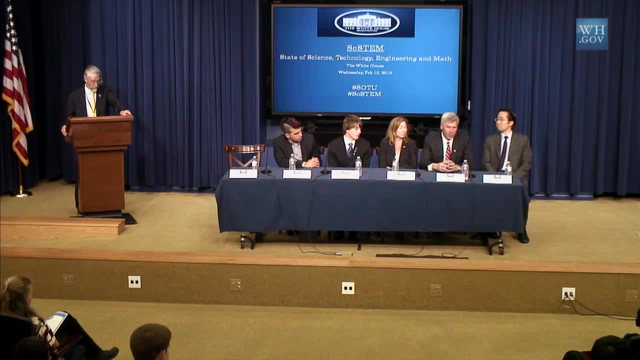 And so when we started iTriage and when I started other companies, it always begins with a big question: So how do you make, how do you solve a very big problem And how do you get started doing that? And that's a big question. 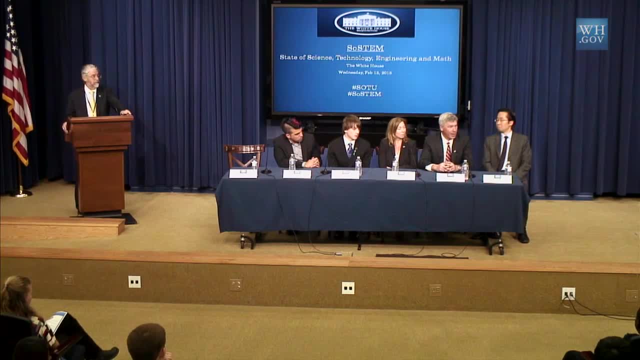 So how do you make, how do you solve a very big problem And how do you get started doing that? And that's a big question. And that's a big question. And then the questions keep flowing after that And, I think, having the diligence to continue to ask. 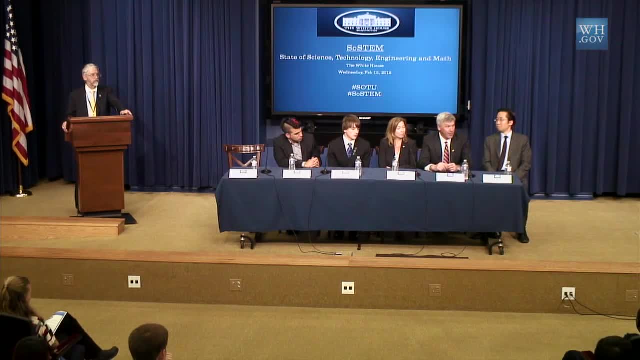 those questions and keep trying to make things better and inventing along the way is how you know new business starts and how technology gets applied in ways that can really make a difference for society and for people in general. Mr Good, Let's see we have a couple in the second row in this section. 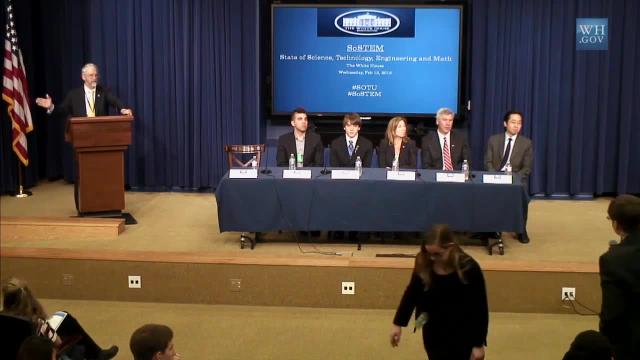 that we ought to hit. Then we'll come back over to the, to the, you know, to the next panel. Hello, I'm Alec Brenner from Thomas Jefferson High School for Science and Technology. Once again, a heartfelt congratulations for the success. 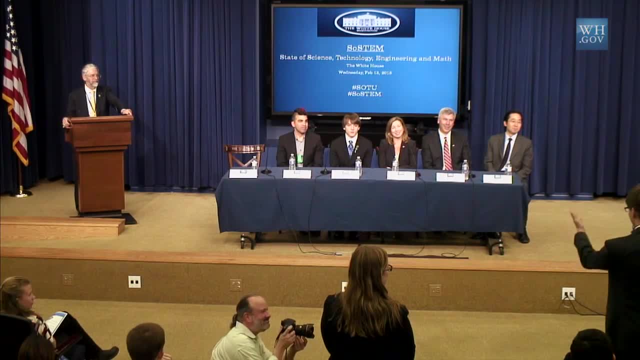 of landing MSL Curiosity, at least half of which must have been due to Mr Friedoski's amazing hairdo. In light of that success, what are NASA's next priorities for space exploration beyond MSL and current space missions? Mr Nick, go ahead. 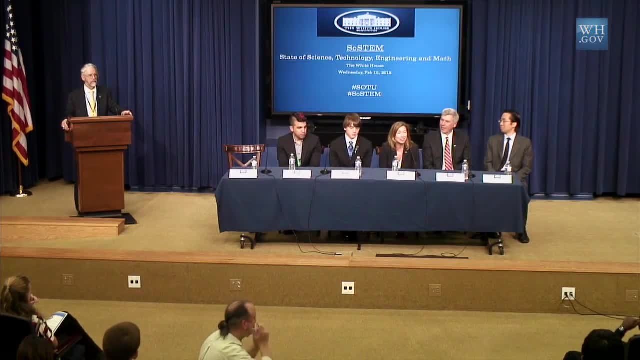 Ms. So NASA is driving to explore beyond the moon's orbit, as Dr Holden said, to an asteroid. That's our next human destination. Right now, with the shuttle retirement, we are really focused on the International Space Station as our foothold to the universe. 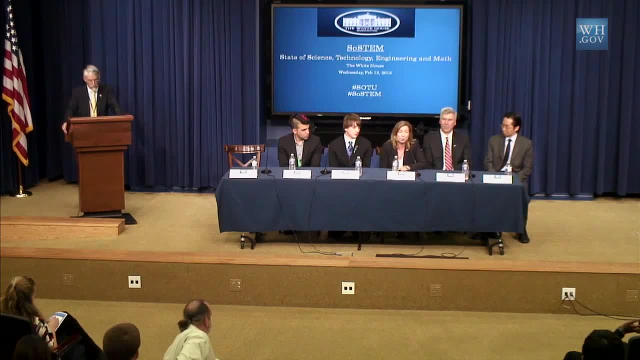 Six astronauts and cosmonauts from four different countries are orbiting overhead as we speak. We have been doing that consistently for 12 years. Just within the last year, 400 scientific experiments on the International Space Station. Astronauts are learning to live and work in space. for those, 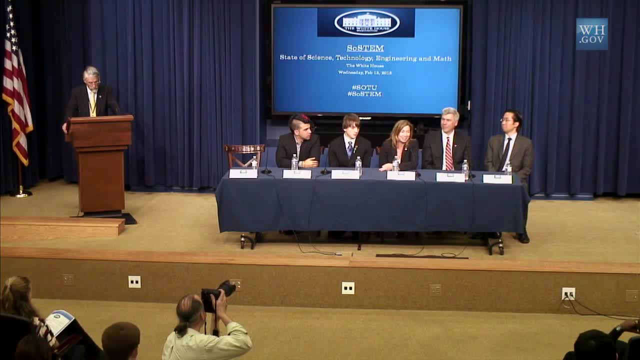 exploration missions to go beyond Again, ultimately to Mars. So Mars Curiosity and the rover- we announced that will happen again in 2020- are precursor explorers to people like you who will be able to explore. We also study a lot of other scientific advancements from the 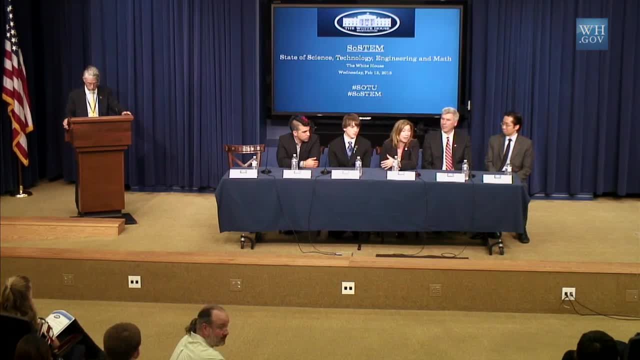 unique vantage point of space Earth science Right now. we had a launch day before yesterday which will be our 17th operational spacecraft looking down at Earth, So we are very excited to be able to do that. We are very excited to be able to do that. 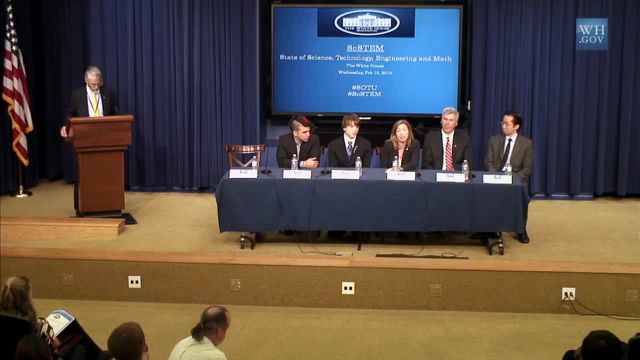 We are very excited to be able to understand this great planet. The President talked about that last night: the importance of being able to protect our planet. It depends on having the best information. So we are explorers out as well as back here on Earth. 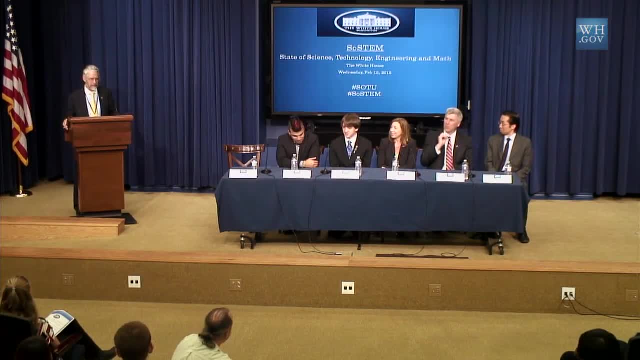 Mr, I'm going to break protocol for just a second. I'm going to ask Jack and Draca a question that I am astonished no one in the audience has asked him yet, which is: how did you come to be interested at such an early age? 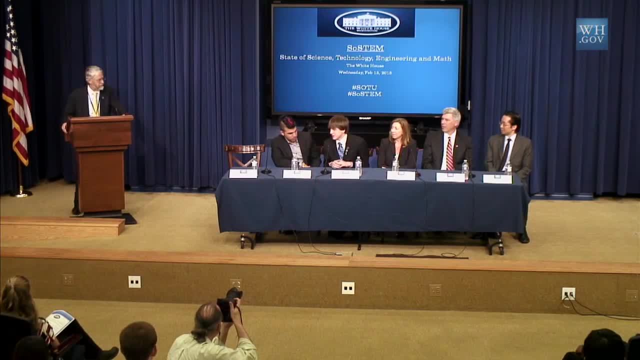 in such an esoteric field as cancer detection Dr. So I actually became interested in pancreatic cancer specifically because a close family friend, who was like an uncle, passed from the disease. And then what I did is I just used Google and Wikipedia and I found that the current standard of pancreatic cancer detection is really lacking. Each test costs about $800 and misses 30% of all cancers, And so I was like I have to do something about this, And so I just used Google and Wikipedia and came up with this. 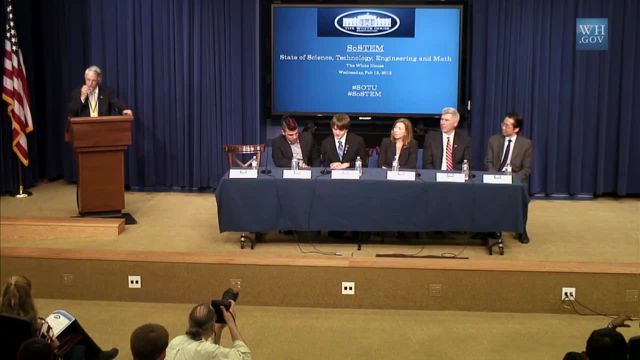 idea to do pancreatic cancer, And so really my big thing is using the Internet for different things and seeing that you don't have to take duck face pictures of yourself or take pictures of your food and post them on Instagram. instead, you could be using it to change the world. 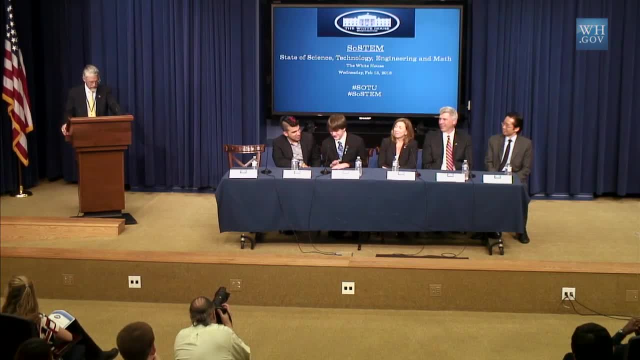 At the beginning of this, I didn't even know I had a pancreas, and so just imagine what you could do. Dr Great, Let's get over to this side again. But anyone who asked a question before I see one young man with his hand up who already had one. 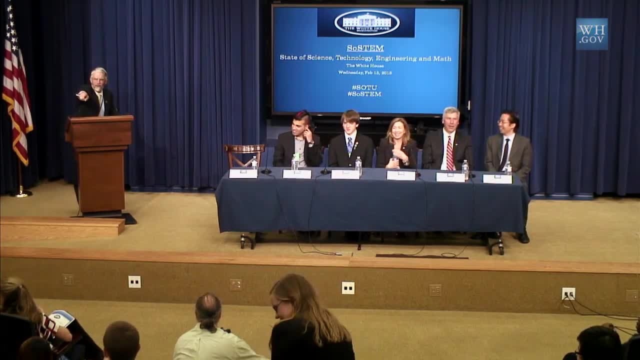 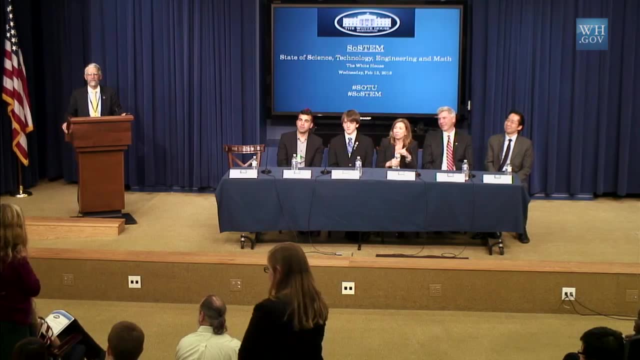 question. nobody is going to get two. We're not going to call on you again Over here in the second row. Hi, my name is Debra Secular and I go to a school without walls. I know earlier you were talking about the intersection of climate. 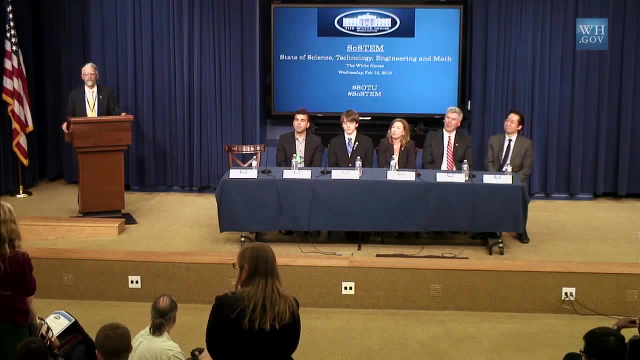 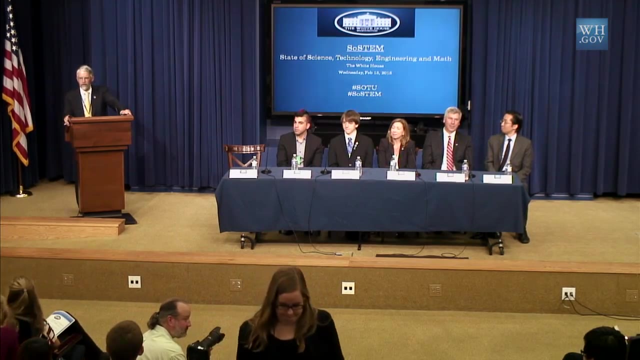 and energy, and I know recently other countries have started implementing carbon taxes or cap and trade schemes and I was wondering if you think a similar measure would have value in the United States and what the political likelihood of that happens, Dr. Well, we know after the first two years of the Obama. 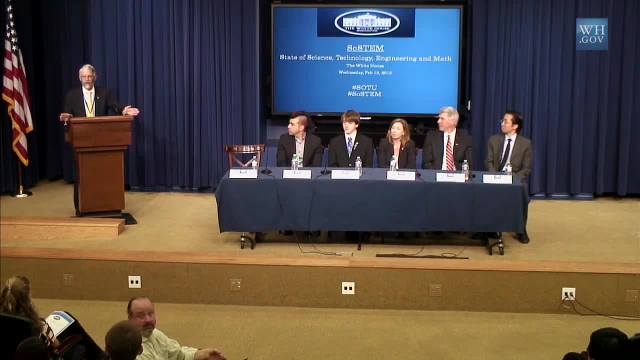 presidency when an attempt to get a comprehensive climate change policy, which would have included a cap and trade scheme, through the Congress failed. it became clear at that point that the best levers against the climate change challenge that were available to the administration were things that 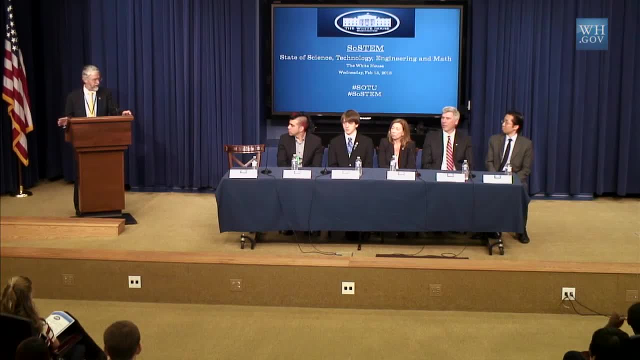 could be done through authorities of executive branch, agencies that already existed, And so the focus has largely been on strengthening fuel economy standards, on encouraging a transition from coal to natural gas and renewable electricity generation, to providing incentives to companies to invest more in clean energy innovation. 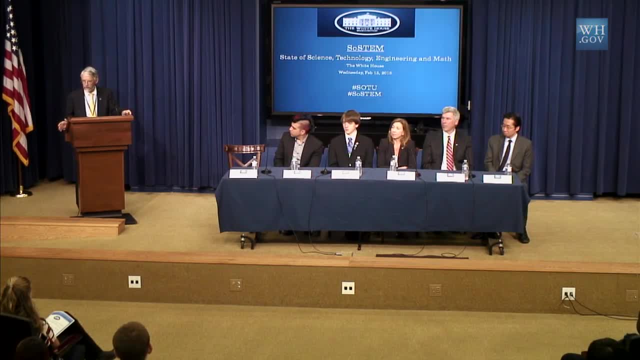 energy efficiency innovation. The President has now, in both his inaugural address and his State of the Union address last night, called on the Congress once more to take action. but he's made clear: if the Congress does not take action, he will continue to act with the executive authorities. 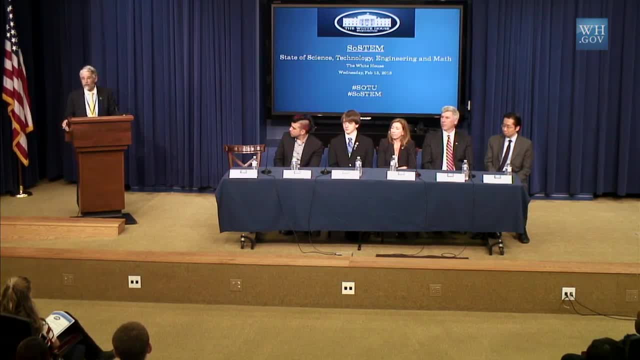 available to him And I think I hope the Congress will take a more comprehensive approach. but I'm not a political odds maker, I'm just a science advisor. In fact, when I get into political odds making occasionally, people sometimes remind me Holdren. 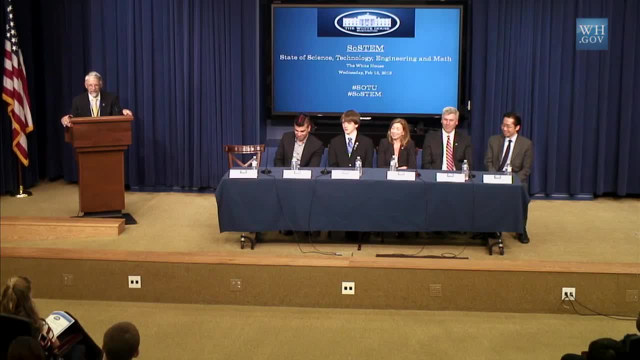 you're just a science advisor. leave the politics to us. So I'm not. I'm not going to try to give odds on what we're going to get out of the Congress, but I will give odds that there will be a wide array of measures that the administration will embrace. 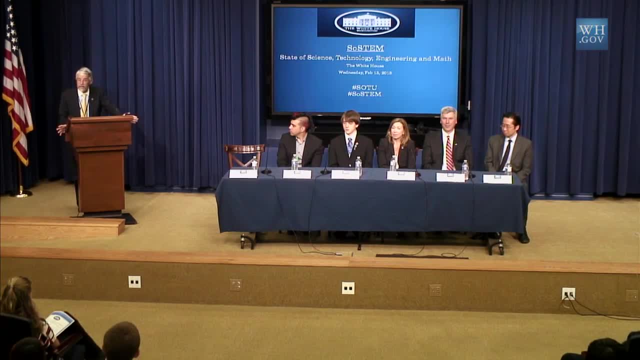 that will advance the ball on the climate change challenge. And, by the way, many of these measures will create jobs and drive economic growth as well, and they will position the United States to be an effective competitor in the global market for technologies that can reduce greenhouse gas. 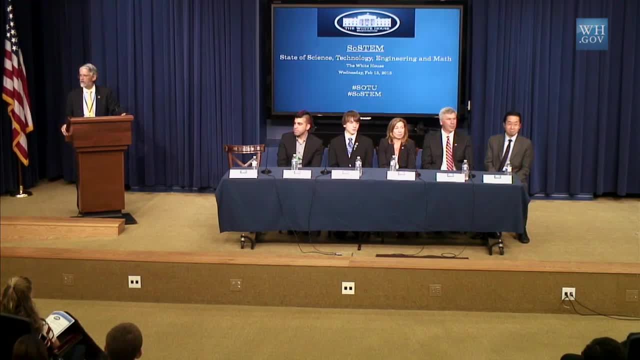 emissions. Let's see where's our mic. Okay, let's go right there. You're in a good position. Hi, my name is Kayuri and I'm from Thomas Jefferson High School. My question is that: how are you guys planning on? 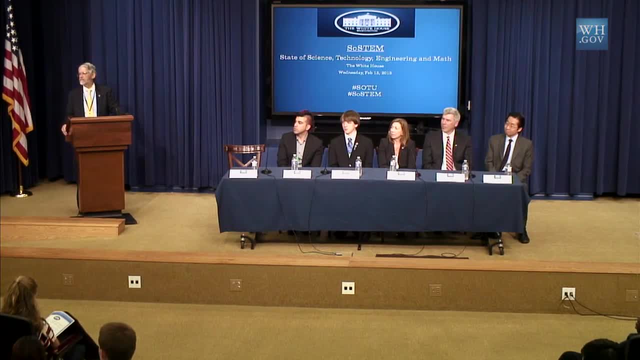 or what has the administration proposed in order to encourage more research past just, I guess, the high school level, but also in college and other initiatives that are going to encourage kids to keep going with research and, you know, make that part of the daily system. 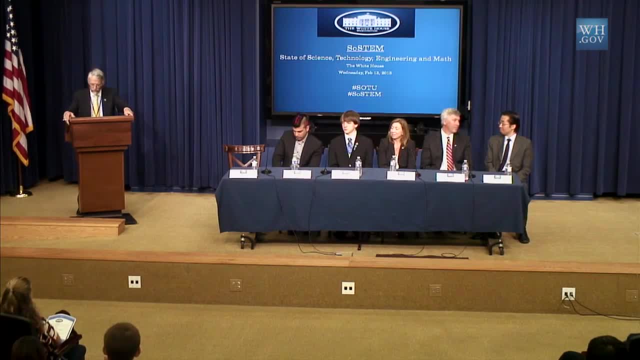 Mr. Okay, that's another big question. We keep trying to keep our answers to two minutes, but we are, first of all, we are doing everything we can in a difficult budget environment to protect the federal government's investments in research and development. 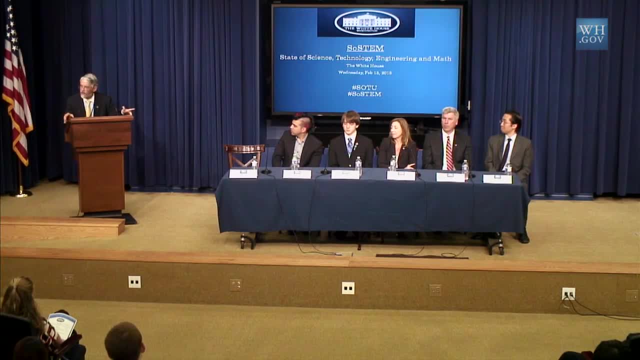 The federal government is the biggest supporter of basic research, fundamental research whose outcome cannot be known and whose gain to society cannot be, you know, established. The federal government is the biggest supporter of basic research, which is what we have predicted, for the obvious reason: 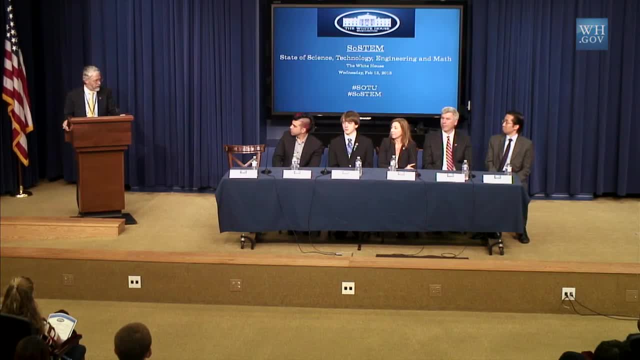 that the private sector likes to invest in things where they have the potential of an economic return. But it's important to remember that the private sector pays for about 70% of all the research that's done in this country, and they do about two-thirds of it. 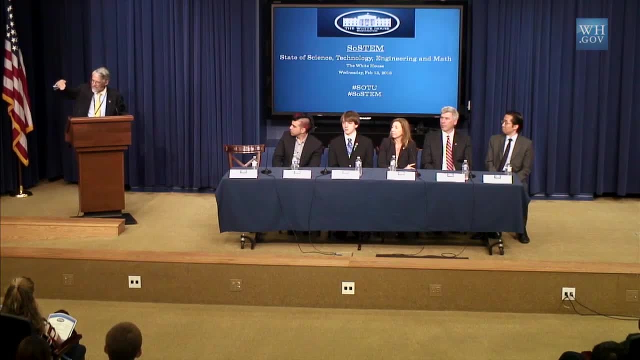 And, as a result, it's not enough for the federal government to maintain or increase, if possible, its own support for research and development. It's important to create an environment that's going to be an environment that encourages the private sector to continue and expand these investments. 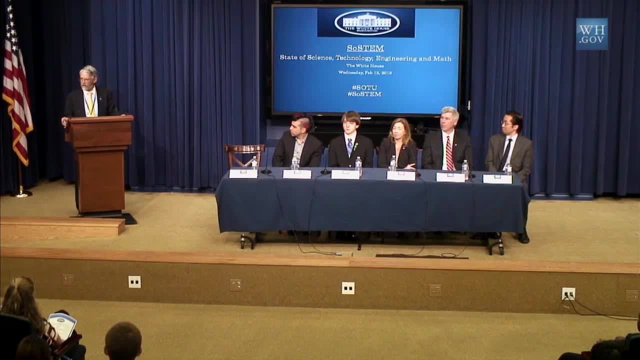 And so we've been working to make the research and experimentation tax credit bigger, simpler and permanent. We've been working to create an environment around patents, around the use of free access to government data, which Todd leads, and a variety of other measures to make this. 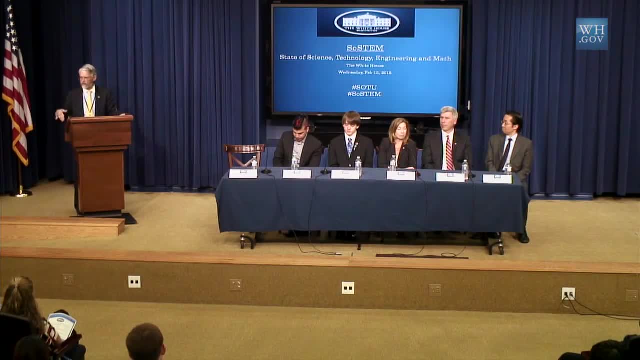 an innovation-friendly society where the private sector will continue to do its part And the jobs and opportunities that are created there in science, technology, engineering and math will also continue to grow, Mr, And just to add a plug for the data part. 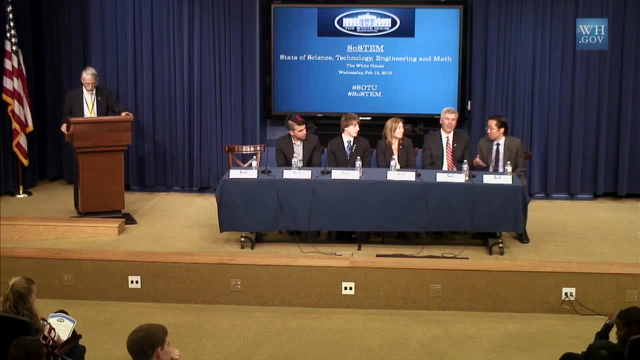 just being the data geek that I am. a key prerequisite to a lot of research is obviously having access to data, And one of the things that the administration is doing, under the leadership of the President, is championing the whole idea of actually making more and more data in the vaults of the 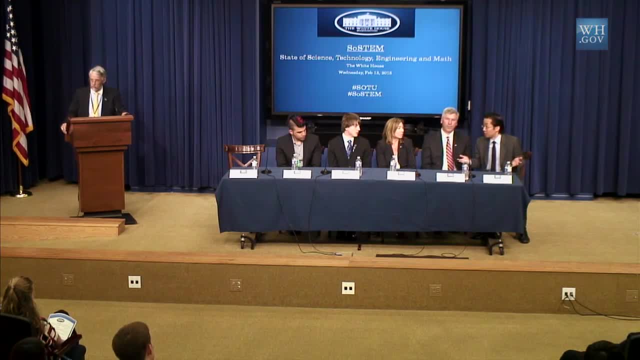 government available, And so the data that we're giving to the public is actually available in machine-level form to anybody for free, So you can actually pick it up and use it to build companies, like Pete has, or pick it up and actually use it to power new. 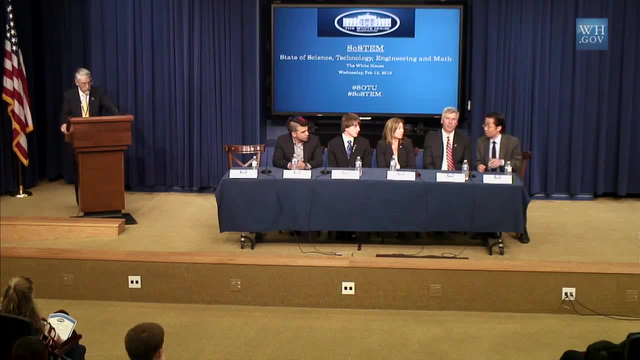 scientific discoveries, And so everyone here in this audience has access now to a massive treasure trove of US government data that you actually, or your parents, paid for and that we're giving back to them and to you. So if you go to datagov, it's got just an extraordinary array. 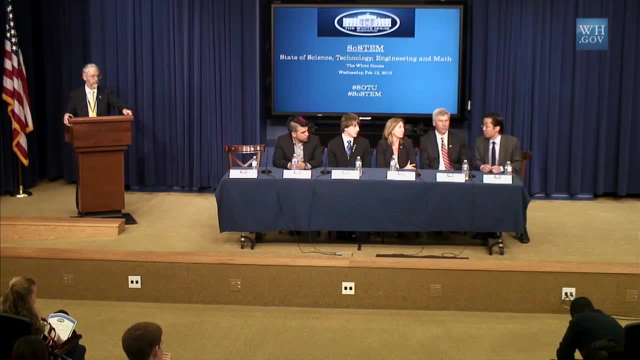 of incredible data resources and can power research at really every level And actually beyond research can actually power development of innovative new products and services and companies like Pete's that have actually created 90 jobs in Denver, saving lots of lives, improving access to health care for all. 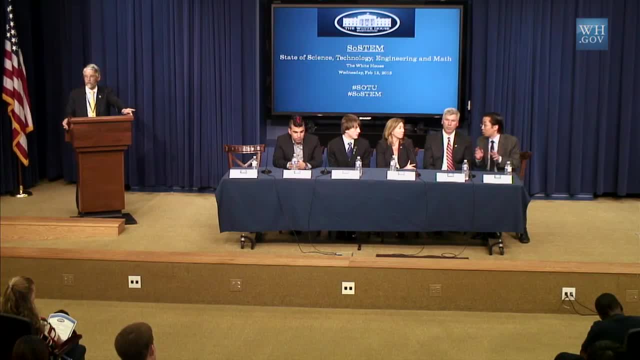 So check it out, datagov, It's your data. You should use it to create awesomeness on an epic scale, Mr, The one further thing I'll mention here is our Grand Challenges effort. I mentioned in my opening remarks the importance of 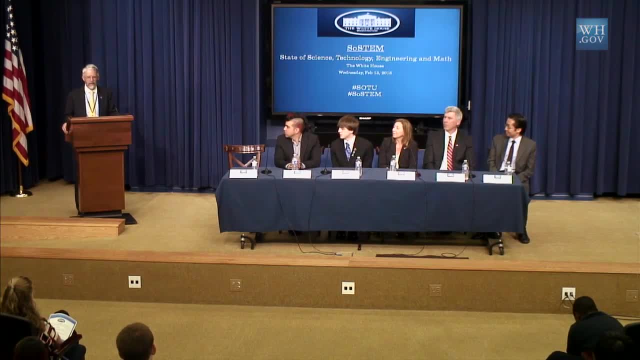 Grand Challenges. Grand Challenges are things like making solar energy cheaper than coal, figuring out how we would deflect an asteroid if one turned out to be on a collision course with the Earth, making batteries that store ten times as much energy as today's batteries. and make electric cars really attractive. 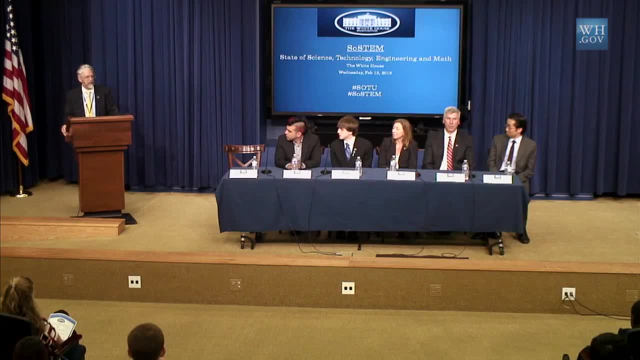 We have a whole Grand Challenges program in the Office of Science and Technology Policy, headed by Kristen Dorgelow- who's standing there in the back- And the focus of that effort is to use Grand Challenges across the public sector, across the private sector. 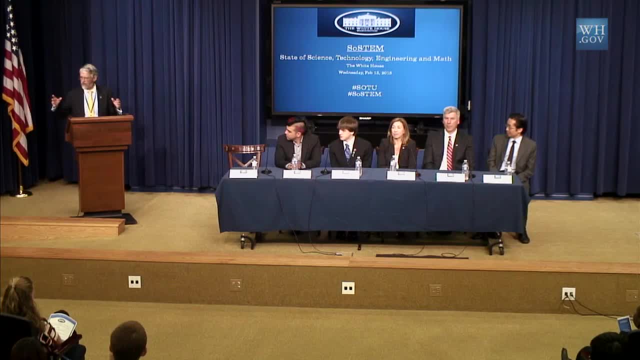 across the academic sector to create more opportunities for people, including young people, to get excited about and contribute to the ways in which science and technology can solve these enormously important problems. All right, Next question: Let's see here. What part of the room have we been missing? 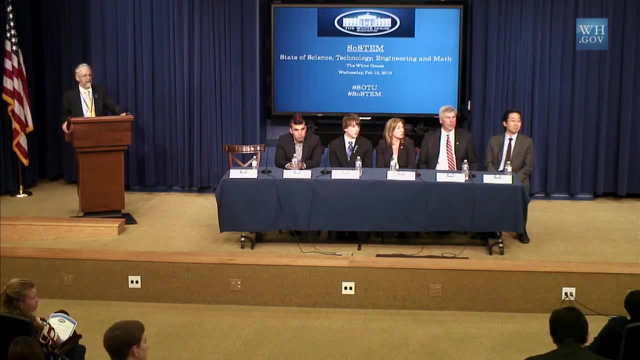 Sort of the back on that side we've been missing. Let's go over there. Hello, My name is Damani Eubanks from Charles Herbert Flowers High School. My question is: with the sequester and other budget cuts, how do you think that will affect STEM research or education? 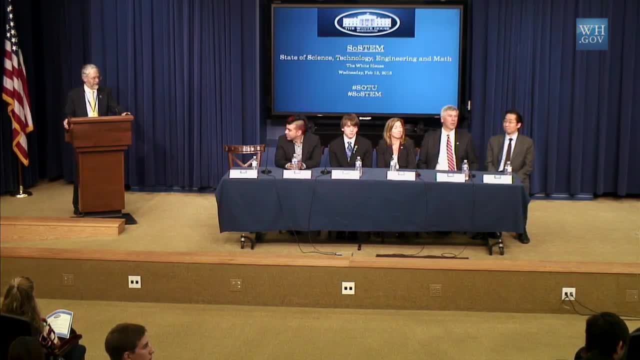 in STEM fields. Mr Gee, Too many of these questions are being lobbed into my court. Some of them have burning fuses on them. Number one: we are doing our best to avoid the sequester and very much hope that it can be avoided. 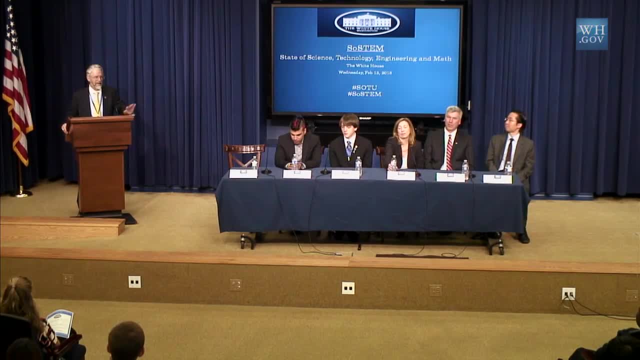 with the cooperation of the Congress, and that we won't have the meat-axe cuts to all of our programs, both defense programs and civilian programs, and including research and development. Those cuts, if they happen, will be devastating. They'll be devastating across the science agencies. 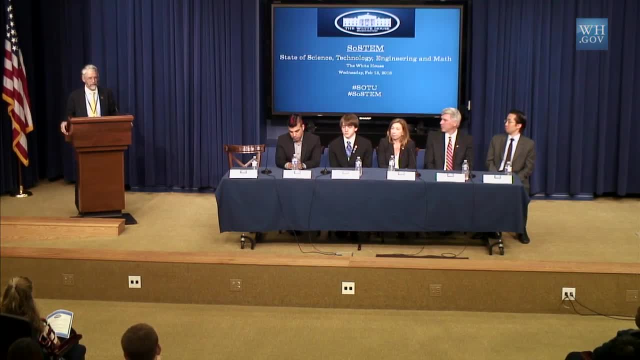 whether it be NASA or the National Institutes of Health or the Department of Energy Science Office or the National Science Foundation. They're going to be devastating and they're going to be harmful to the economy. They're going to be harmful to employment. So the job one is to avoid that happening at all. 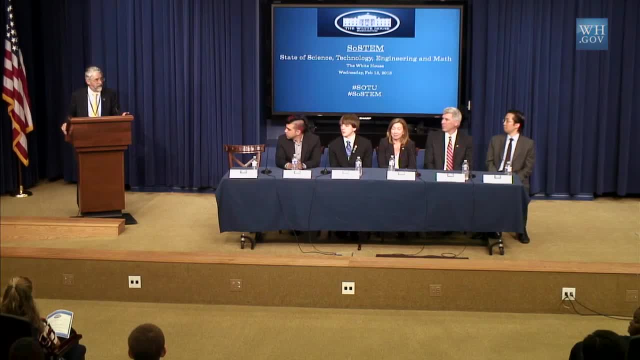 The President has made very clear. he made it clear again last night in his State of the Union speech that cuts that affect education, cuts that affect our investments in science and technology are cuts that are undermining the future of the country. We ought not to be doing that. 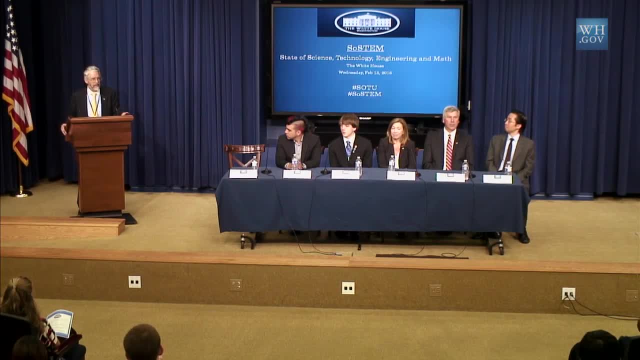 It's not a sensible policy. If, against all reason, the sequester occurs, we obviously will do our best to minimize the impact of the cuts that occur and to minimize their duration in terms of their effect on our research and development enterprise and on. 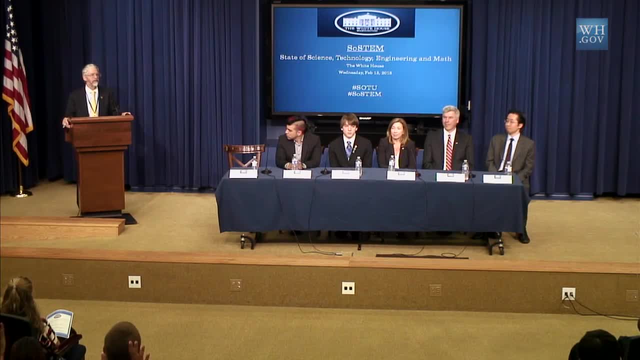 our STEM education enterprise. All right, let's go a little further back on that side, because I don't think we got that part well represented yet. Leila Nasser, Girl Scouts. Hello, I'm Leila Nasser and I'm representing Girl Scouts. 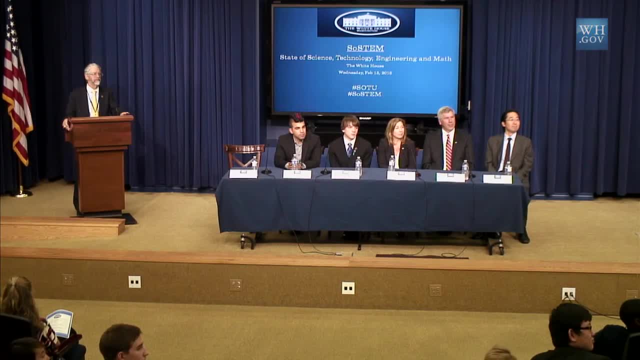 So my question is: is there a way to reduce the number of cuts on the STEM field? My question is: what is the administration doing to encourage more girls to get involved in the STEM field? Ah-ha, this is actually a great topic. 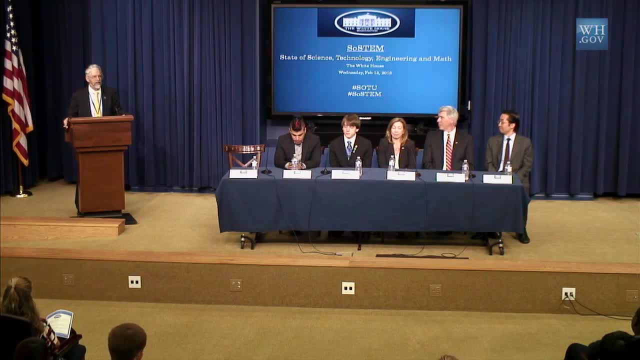 We have a White House Council on Women and Girls that's headed by Tina Chen, who is also the Chief of Staff to the First Lady, And OSTP, in fact, is working very closely with the White House Council on Women and Girls. In fact, our lead person for the White House is a woman and a 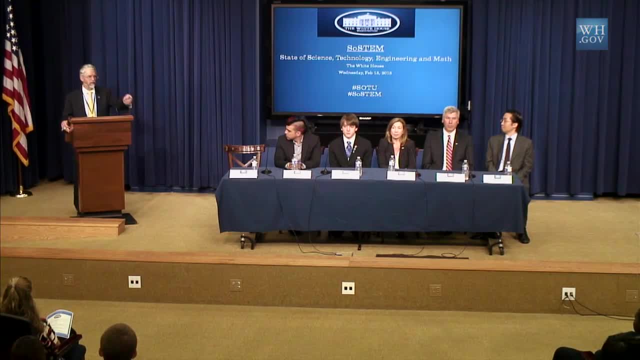 man. The lead person responsible for that is also in the room- Lauren Anderson, who is in the back corner. We've had a wide variety of events around improving opportunities and inspiration for women and girls in STEM fields. The NSF launched more than a year ago a major initiative. 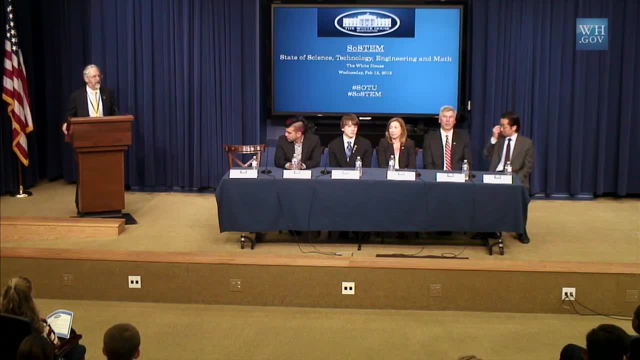 making the conditions of work better for women in science fields who have NSF grants. We have brought a wide variety of leading women scientists and engineers into the White House to inspire audiences like this one with what they've been able to do, and they've been able to. 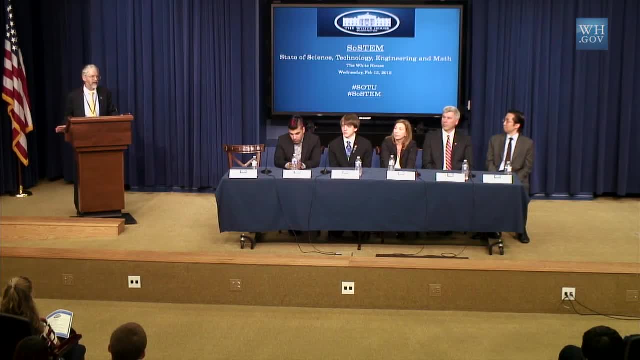 achieve and with their ideas about how to improve access, opportunity and quality of professional life for women and girls in this domain. So this is really a favorite theme here in the White House, one that's very important to the President, very important to the First Lady. 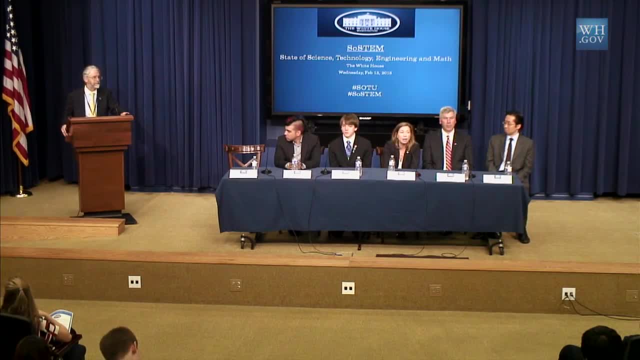 and very important to those of us who work with them. And I'll just add- because we happen to have the head of the NASA STEM Council on Women and Girls in the room too- to Rebecca Spite-Keyser is the director of the NASA program. 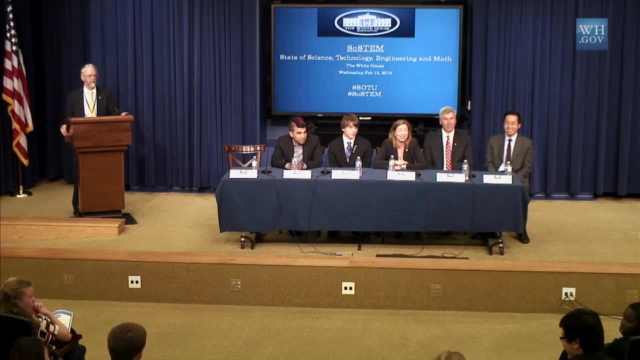 And she is here with her daughter, Sydney, Sydney. I'm going to give you a shout out as well At NASA. this is because I only have sons. it's not fair. I get to adopt Sydney every now and then. This really is a priority. 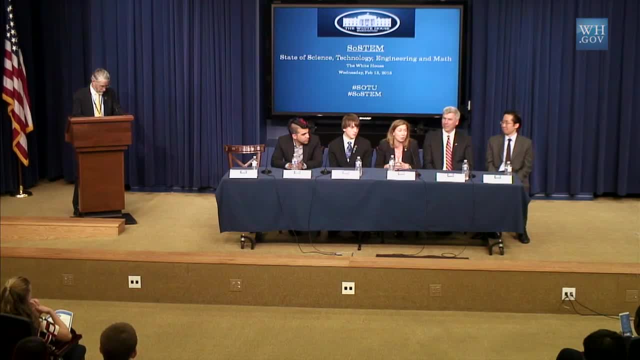 Even at NASA, we have a quarter of our STEM workforce is female And, as I like to point out, we have a lot of female students And, as I like to point out, are we a quarter of the population? No, no, We have more work to do. 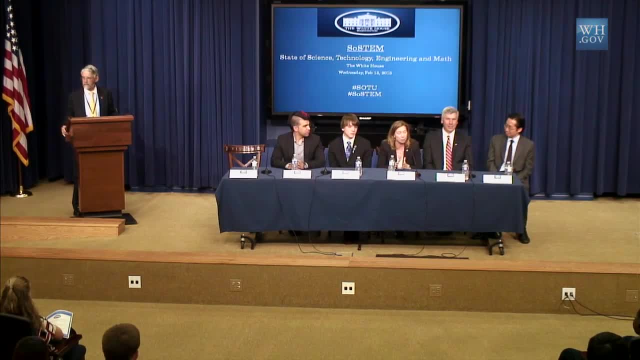 We have within this program and the incredible leadership of the White House. Valerie Jarrett and the First Lady have been working to, as Dr Holdren said, put an emphasis on it in the way that, as we give grants being more aware. 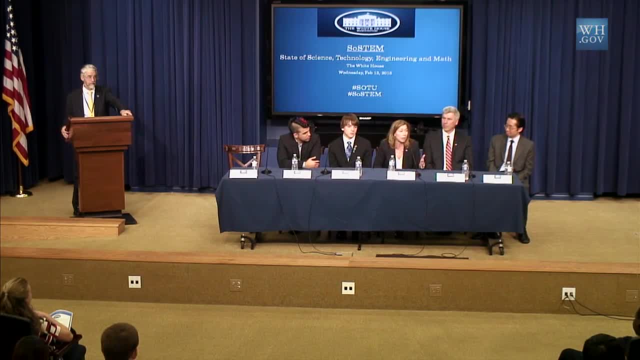 being able to identify role models, And we have a website I would encourage you to go to at NASA Council on Women and Girls. Thanks, Thank you, Valerie. Okay, We have some back row from the right side of the room. Hi, I'm Juliana Bain. 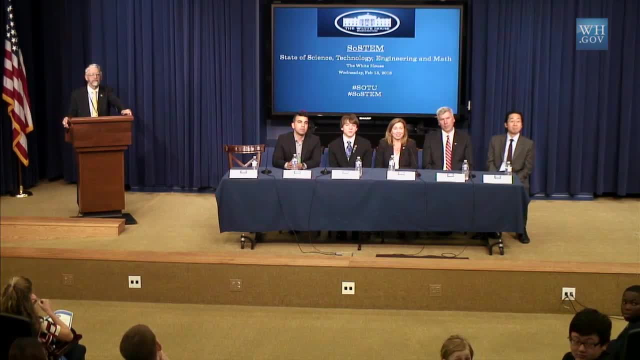 I go to Thomas Jefferson High School for Science and Technology And I'm Lucy Binslinger from HB Woodlawn High School. We have a question for Jack. How did you test the effectiveness of your pancreas cancer sensor And, after your research, how did you even get started with coming? 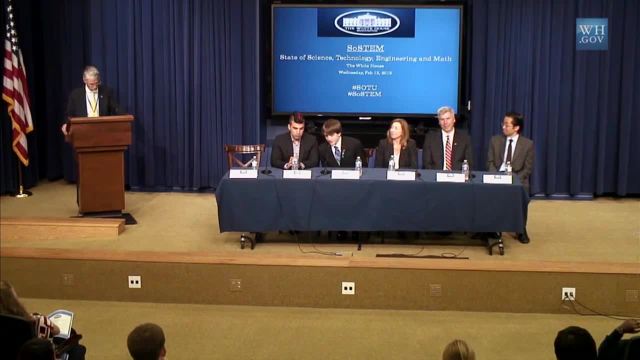 up with your cancer test, Dr. So I'm a PhD student. I'm a PhD student, So essentially what I did for after I created the sensor, that actually took me quite a long time. It took me five months, like over, like my deadline. 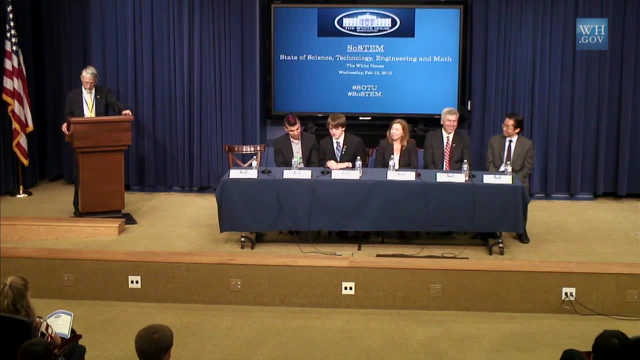 So, but in order to test the effectiveness of the sensor, essentially what you do is first you test mouse samples, And so they have pancreatic cancer samples in them, And so they have the mesothelium protein, which is the cancer biomarker I was looking for. 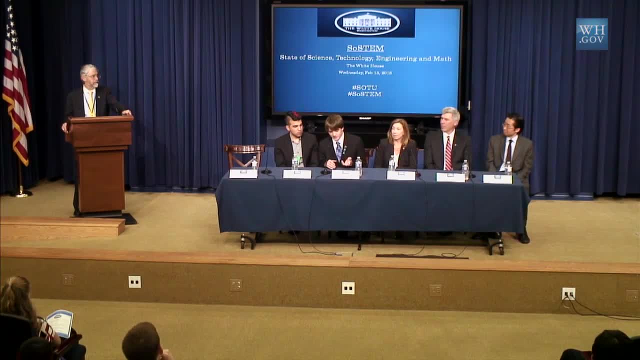 already circulating in their blood And so essentially I took blood samples and I tested them And it just requires a 6th of a drop of blood, so it was extremely noninvasive to the mice. For all of you animal activists out there, 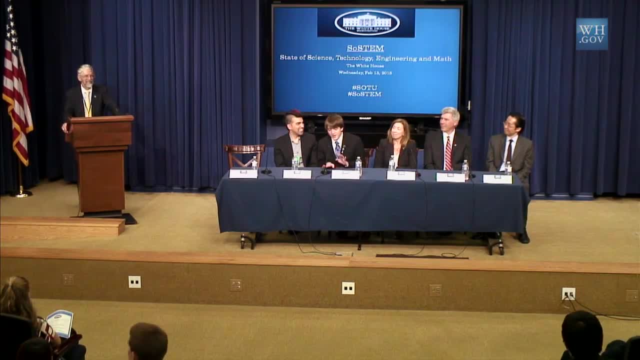 they didn't feel that much pain. And then so after I did my research, essentially what happened is I actually did all my research from my house, like on the background research, And then I wrote an e-mail- actually 200 e-mails. to the National Institutes of Health and then also So the Johns Hopkins University, and out of those I got 199 rejections and one lukewarm maybe, And I actually had to go through three months of phone tag with the professor to get into his lab. But eventually I did, and seven months later I had one small paper sensor that had 100% accuracy. Wow, Okay, we have time for two more. I'm going to apologize preemptively to those who missed. There's a gentleman in the second row here who's going to get one of them. 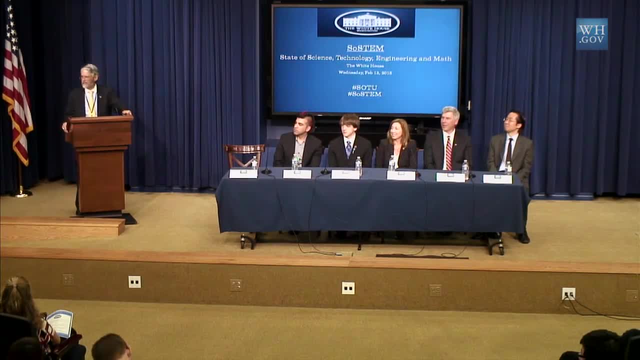 and then the woman in the third will get the young woman and the third will get the other. My name is Vincent DiPerna from Glasgow Middle School, And do you think that we should have solar panels on the highest buildings in downtown areas? required? 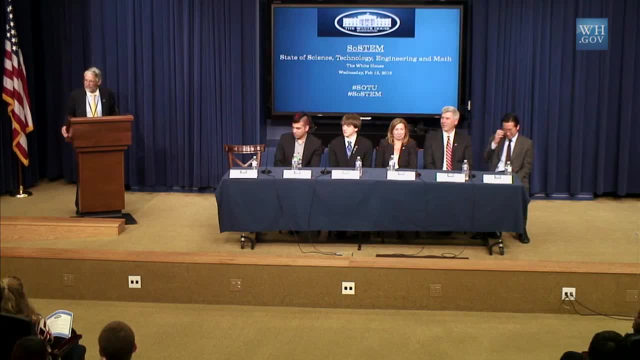 Question: should we have solar panels on the highest buildings? Well, I think we should have solar panels everywhere, that they're economical. And again, we've been making great progress. Solar panels have been getting less expensive. If we just project current trends, they will become less expensive than fossil fuels before long. 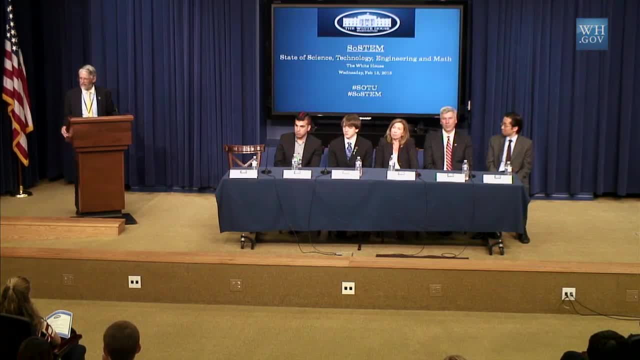 And I think we will see solar panels on a lot more buildings- tall ones, short ones, medium-sized ones and also in arrays- And I think that we should have solar panels on the highest buildings in downtown areas required. There's a big future for solar energy in this country. 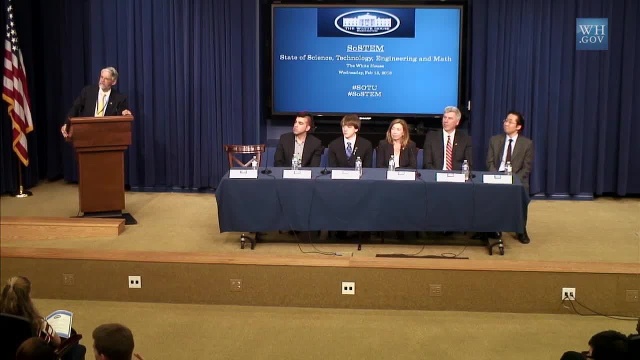 Now in the young woman in the third row. Hi, Dr Holder. My name is Thersha Potleri from Thomas Jefferson High School for Science and Technology. I talked to you earlier this year when you visited our school And we took a tour around the school facilities and you visited our energy systems lab. 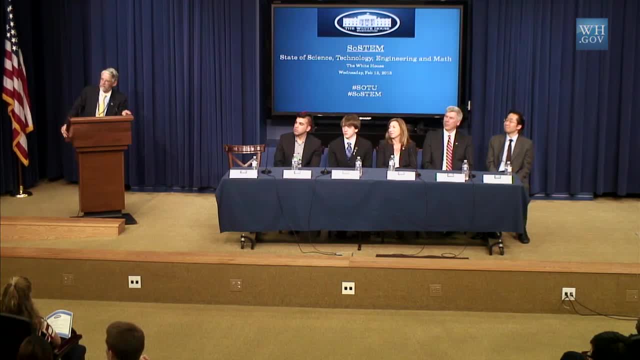 And we have a project where we're launching a satellite in collaboration with NASA, actually later this year And then later in your community, we're going to be launching a satellite in collaboration with NASA And then later in your community, we're going to be launching a satellite in collaboration with NASA. 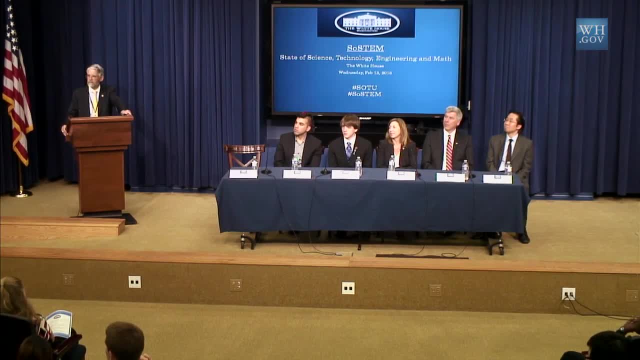 keynote speech, you mentioned increased collaboration between the government and high school students, And so we were wondering. my question was: with President Obama's second term, how is the Obama administration working to increase this collaboration between students and the government? Mr, Well, that's actually a great question. 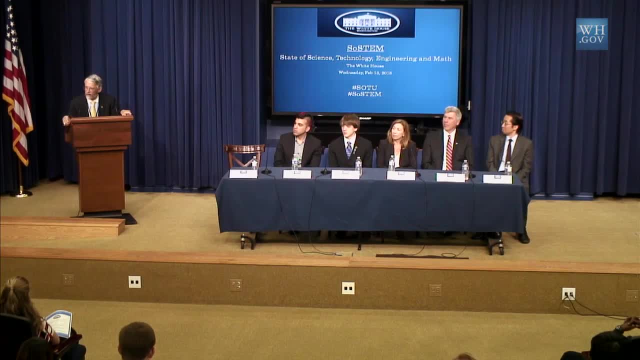 Obviously, we're very early in the second term and we're having a lot of conversations about how we're going to use the opportunity of another four years of the Obama administration to advance the ball in all these STEM fields, And that will certainly include working with high school and 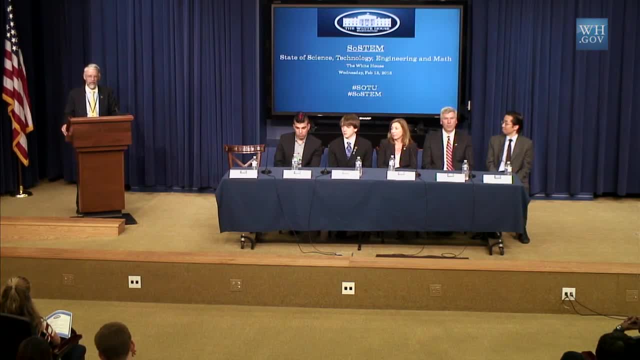 with middle school students. I think we'll be seeing more science fairs, We'll be seeing more efforts to find ways to get high school students certainly- and maybe middle school students- involved in real world research problems. I think some of the efforts that have been mentioned already in 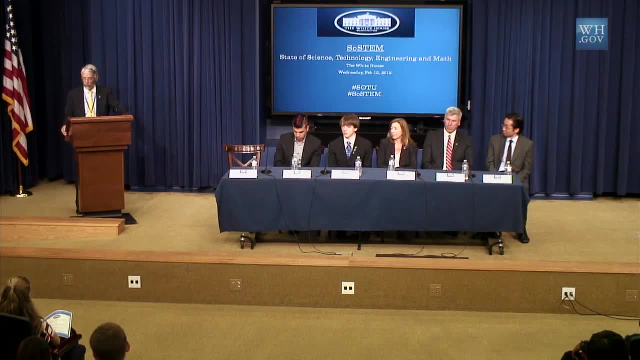 terms of how we get more women and girls interested in and involved in science are going to certainly be pushed forward very hard in this administration, But we're really not done. thinking about this And I think you have my e-mail address. I will welcome your further thoughts about what we might be. 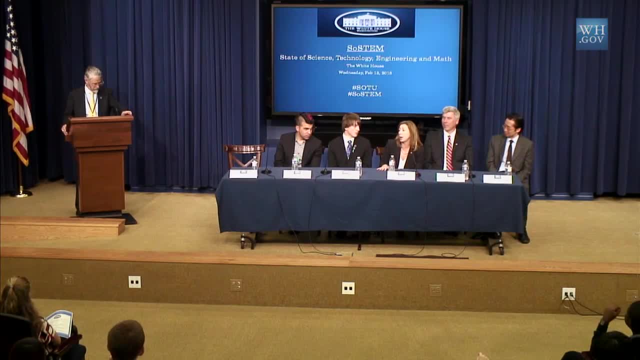 doing that. we're not, Ms. I'll give you one specific example as well: We're expanding, certainly in the second term, a program where you can online high school students put forward experiments that the winners will be flown on the International Space Station. 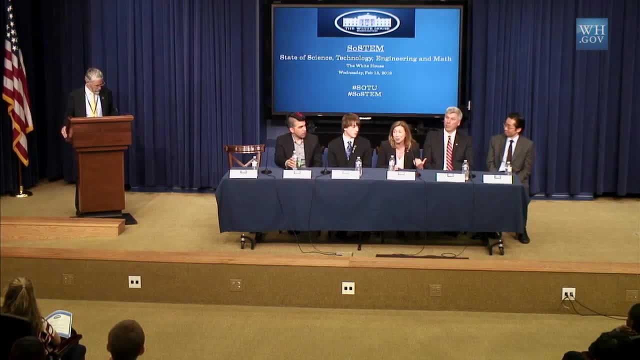 We just closed one round, but we'll be expanding it And that is a program that is sponsored by the private sector. So it's a great partnership opportunity and we'll be expanding those, Mr, And I'm hoping that the achievements like those of Jack. 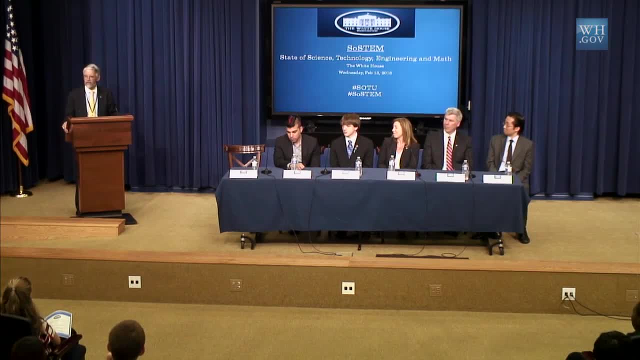 Andrejka and other young people who've made astonishing contributions to science and technology at an early age, will lead to a situation that when one of you sends out 200 e-mails asking for access, that you'll get more than one tentative lukewarm acceptance. 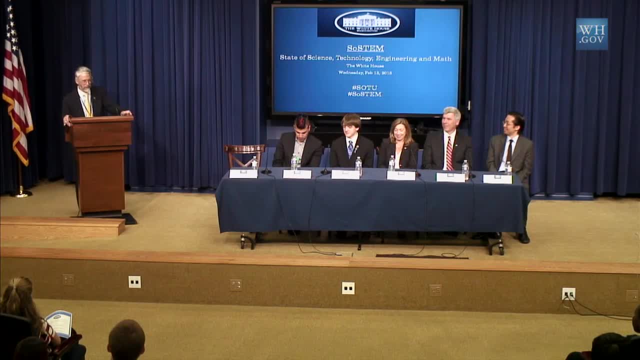 Maybe 100 acceptances would be an appropriate ratio. So, again, inspiration is part of this, and inspiration works two ways. We hope that the success of folks like the folks at the table here will inspire you, but I also want you to know that you 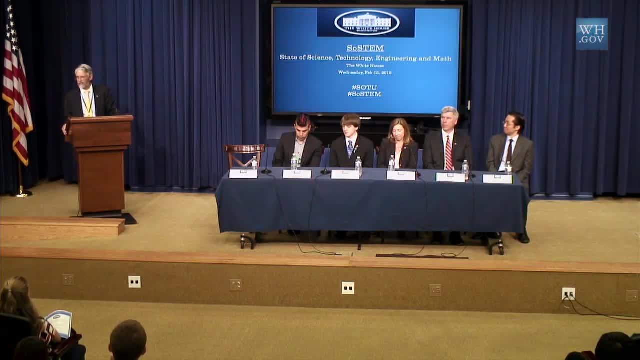 inspire us, and your ideas and your energy are one of the reasons we have such high hopes for the future. So with that, let me thank you all again for being here. Let me thank Bess Evans and all of her team, our folks in the Office of Public Engagement and our folks. 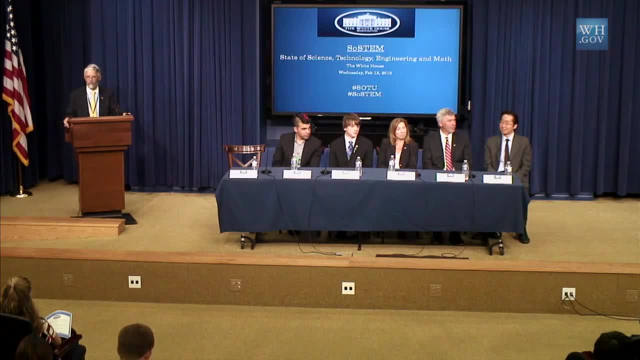 in OSTP who made this event possible, But above all, thanks to you, young people, and your teachers, your mentors and your parents, because you are the future, And I should have thanked our extraordinary panel for devoting their time to answering these amazingly perceptive questions. 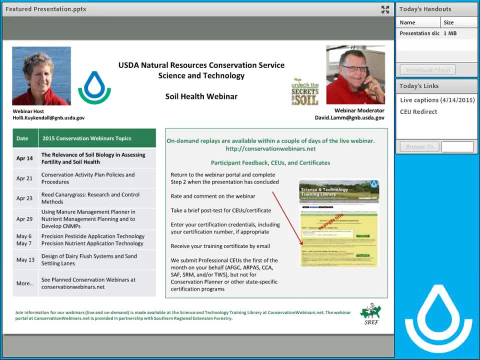 Getting started with our soil health webinar today, again, I'm Holly Kirkendall, webinar coordinator for NRCS's East National Technology Support Center. I'm pleased to turn the webinar over to our moderator, David Lamb. David is the leader of the National Soil Health and. 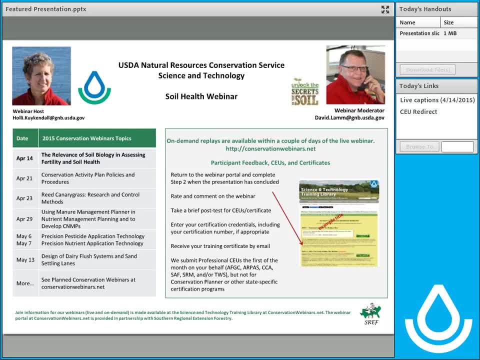 Sustainability Team here at the East National Technology Support Center in Greensboro. David, you may now begin, David Lamb. Thank you, Holly. Again, this is David Lamb, and I'm actually sitting in Ames, Iowa, and teaching a course that NRCS offers called. 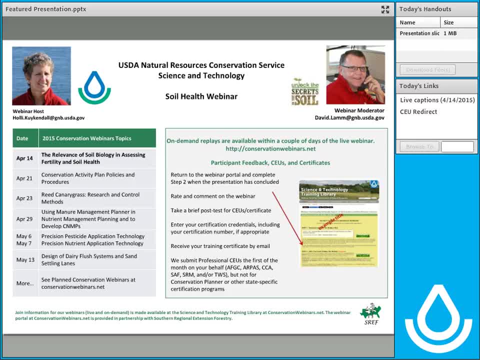 Soil, Health and Sustainability for Field Employees. and we're trying something new today: We're actually using Dr Brenton's live webinar presentation as part of our course presentation. So not only am I here sitting in my room, I've also got 32 or 34 NRCS employees that 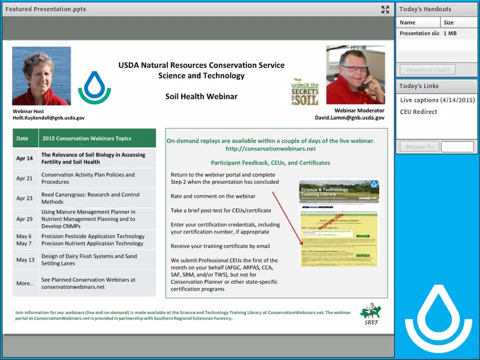 are participating in the course, So let's tackle that. It's kind of exciting being able to take advantage of this technology. Let me introduce Dr Brenton. It's been my privilege to know Dr Brenton, or Will, for the last four or five years since. 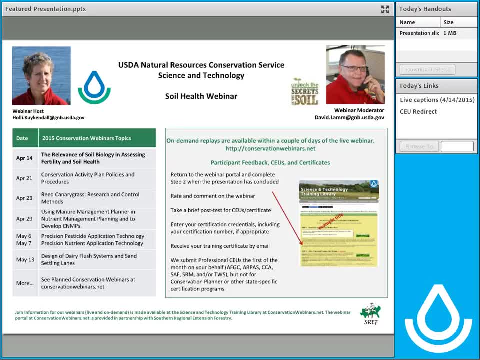 I've been involved with soil health. Dr Brenton is a native of Pennsylvania and he attended agricultural school in Chester County and in Barnesville Ohio. He managed a 20-acre organic vegetable farm for several years while he was attending agronomy school in Maine.